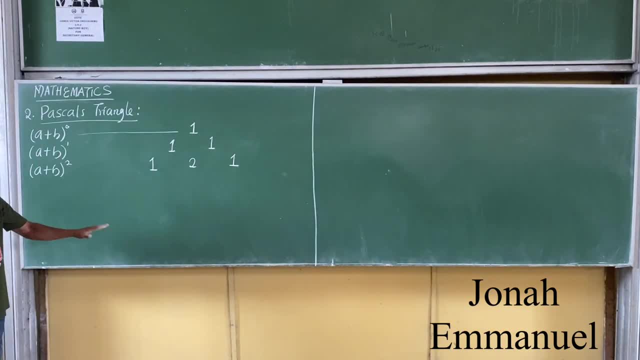 So I'm adding 1,, 2,, 1.. If I'm considering to the power of 3,, I add a plus b to the power of 3.. The rule says it starts with 1.. The term in the tree is got by adding the two previous ones. 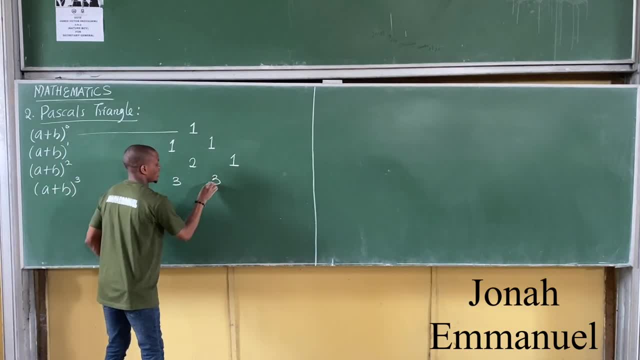 1 plus 2 gives 3.. 2 plus 1 gives 3.. And I'm adding 1.. I'm adding 1,, 3,, 3,, 1.. We'll take one more, 2, to the power of 4.. 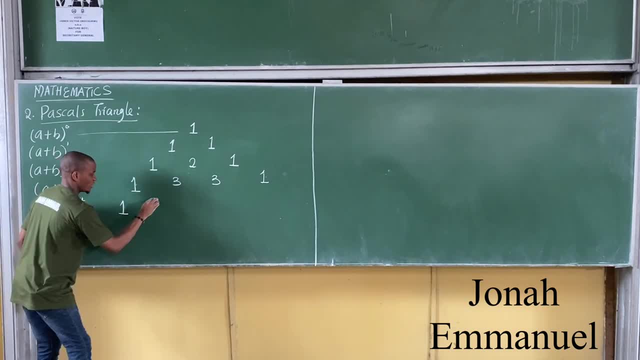 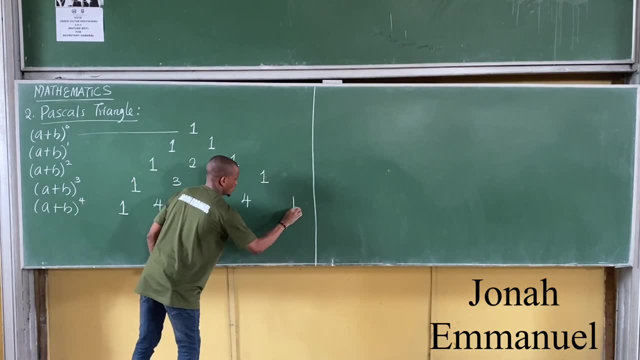 So I'll start with usually 1.. 1 plus 3 gives 4.. 3 plus 3 gives 6.. 3 plus 1 gives 4.. Ends with 1.. So I have this. I'll take a few more. 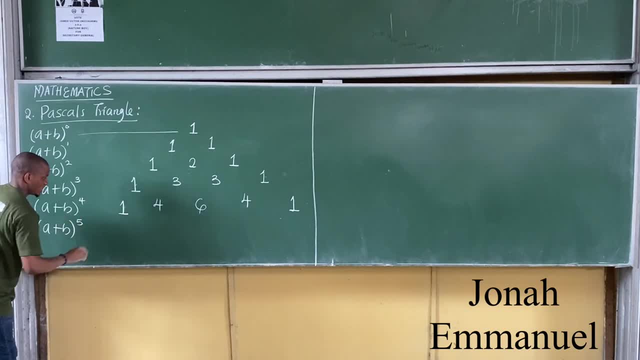 I'm adding a plus b to the power of 5.. That gives me 1.. 1 plus 4 gives 5.. 4 plus 6 gives 10.. 6 plus 4 gives 10.. 4 plus 1 gives 5.. 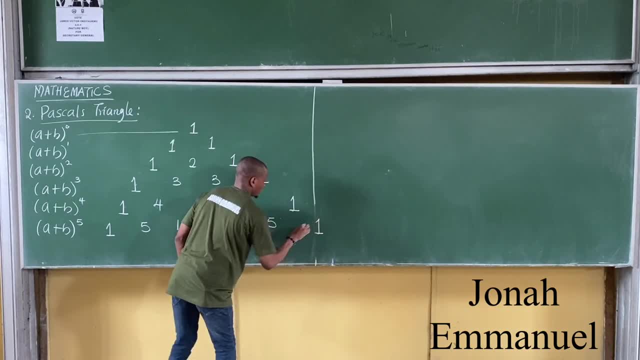 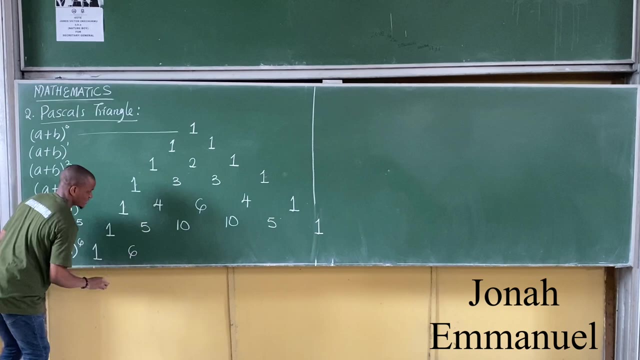 And I have 1 here, So I have 1.. Let's take one final One, final 10.. a plus b to the power of 6.. So this becomes 1.. 1 plus 5 is 6.. 5 plus 10 is 15.. 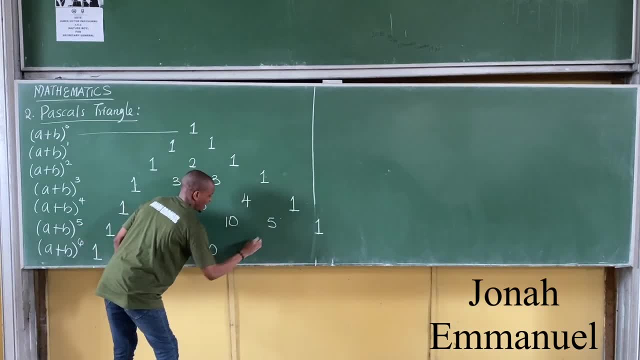 10 plus 10 is 20.. 10 plus 5 is 15.. 5 plus 1 is 6.. 10 plus 1.. All right, So this is the Pascal's Triangle coefficient for degree 0 to 6.. 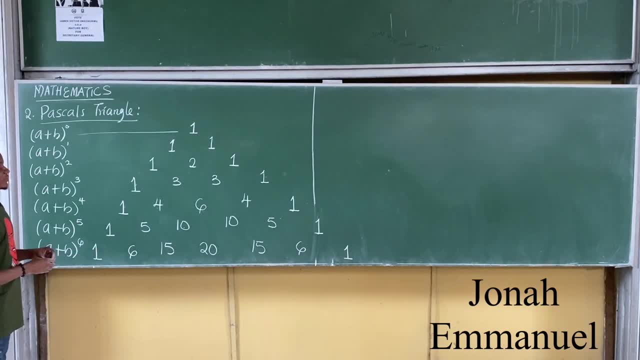 So I have this there. Now this is called Pascal's Triangle, because if I put this up like this, you can see it forms a triangular shape. It forms a triangular shape. You can see here. I'm adding this down here, So I'm going to go this way. 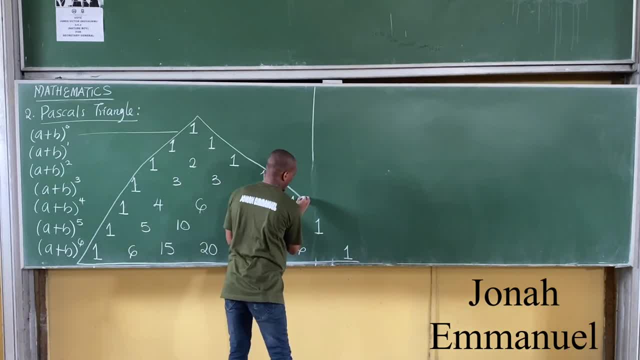 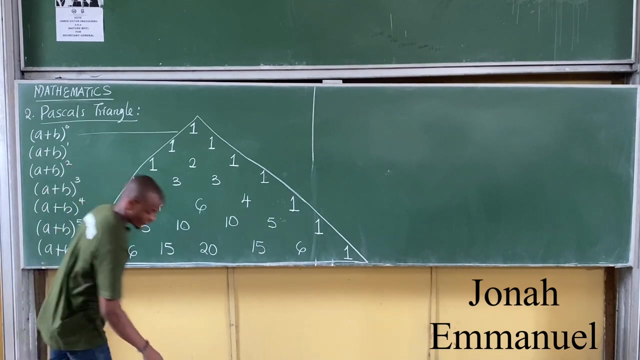 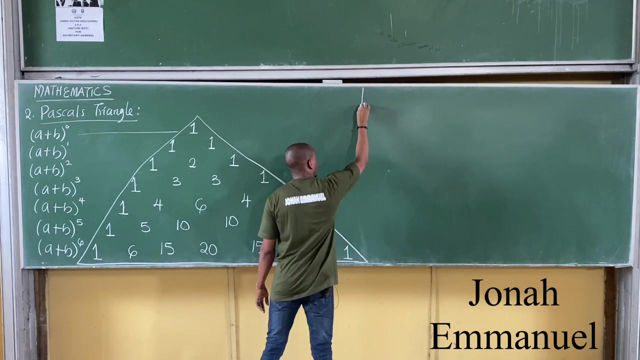 I'm adding this down up to this. All right, So it forms a triangular shape, A triangular shape That is called Pascal's Triangle. We'll see how it applies to the Pascal's Triangle to solving problems of binomial expansion. We'll see how it applies to the Pascal's Triangle to solving problems of binomial expansion. 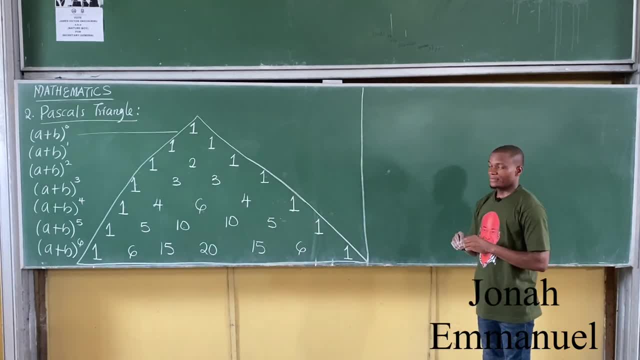 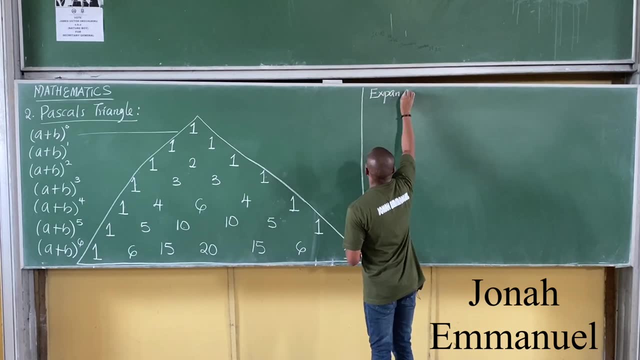 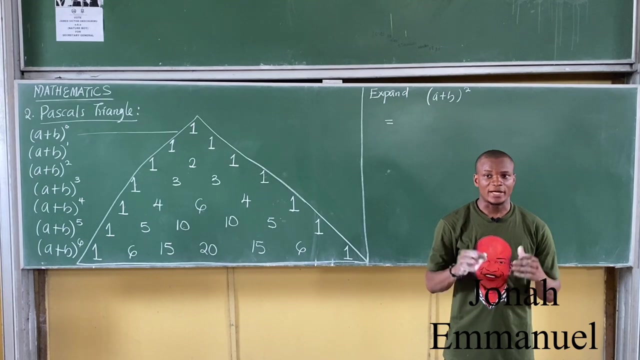 All right, Let's take some examples. Let's take some examples. Let's say we're going to expand. Let's say we're going to expand this a plus b to the power 2.. All right, Using Pascal's Triangle. Let's say we have to expand a plus b to the power 2. using Pascal's Triangle: 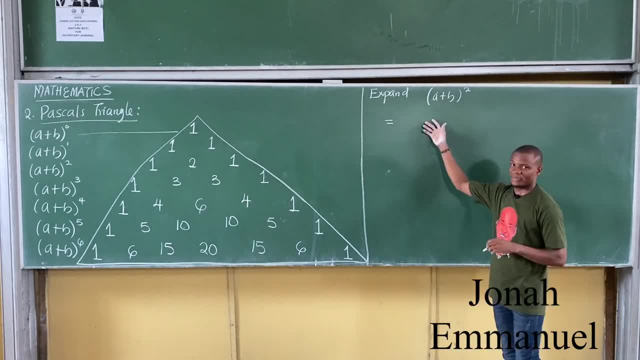 All right, In our previous class we expanded this using general expansion method. But how do we expand this using Pascal's Triangle? Now, here's the concept for Pascal's Triangle, Case 1.. Case 1. Here's how you start. 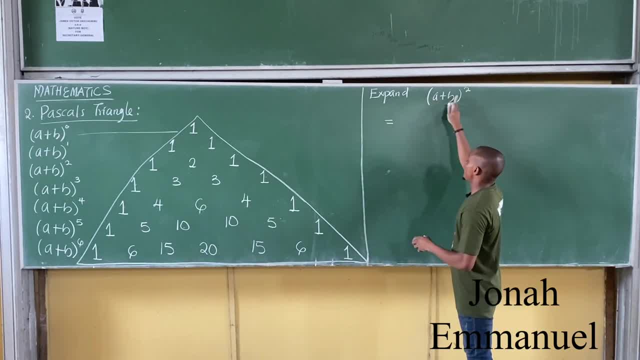 The first term takes all the power. The power there is 2.. So I have a to the power 2.. Of course, if the first term takes all the power, the second term is left with nothing. It becomes a to the power 2, b to the power 0.. 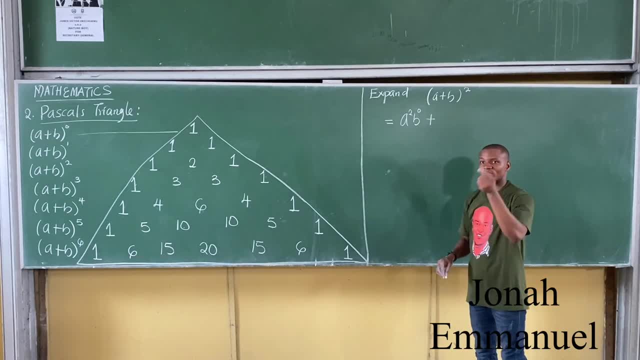 Plus for my next term. I will decrease the power of the first term by 1. And I will increase the power of the second term by 1.. All right, So the concept is this: Decrease the power of the first term by 1.. 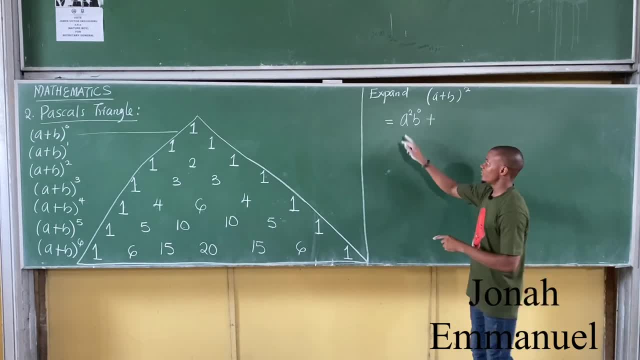 Increase the power of the second term by 1.. So I'm having a here, The power there is 2.. Reduce it by 1. It becomes 2 minus 1. That's 1. B. Increase this by 1.. 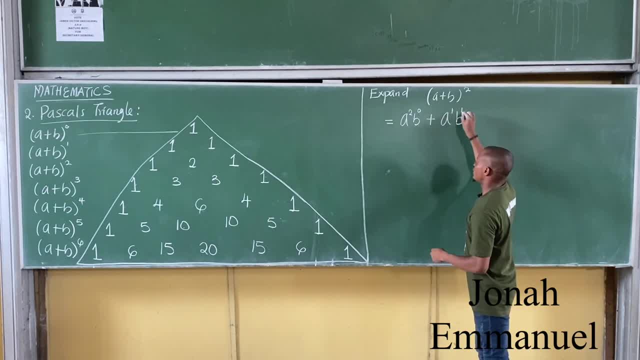 To become 0 plus 1 is 1.. So I'm having this Plus. that same concept continues My first term, a: Reduce the power by 1.. Reduce the power by 1. It becomes 1 minus 1, which is 0.. 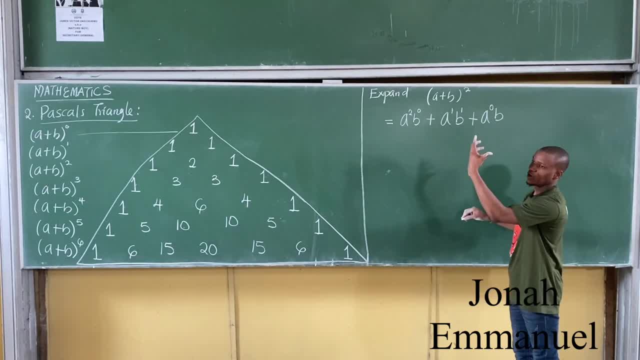 For the second term. you said: increase the power by 1. It becomes 1 plus 1.. That gives you 2.. You stop at the point where I'm having the second term bearing all the power. So it becomes this. So I'll stop at this point. 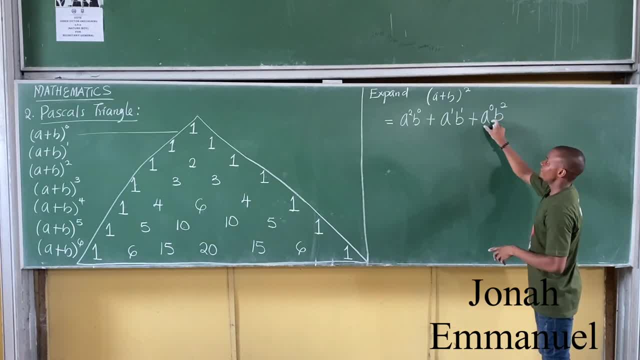 Why am I stopping here For my last term? the first term will be to power 0. And your second term will be to all the power, So I'll stop here. This is now equal to: This: gives you a squared a to the power 0 gives 1.. 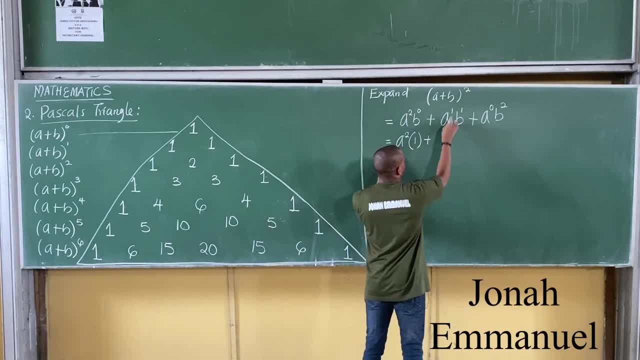 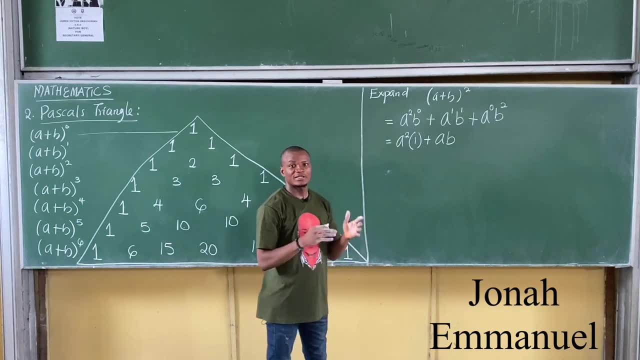 From the 0 to the p basis, Plus a to the power 1 is a, b to the power, 1 is b. Usually, when a number is a to the power 1, it becomes that same term. That's the concept. 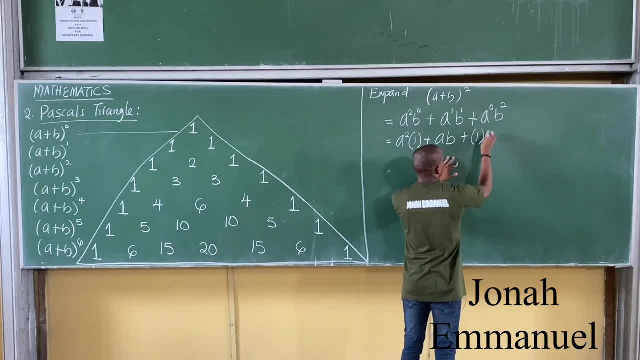 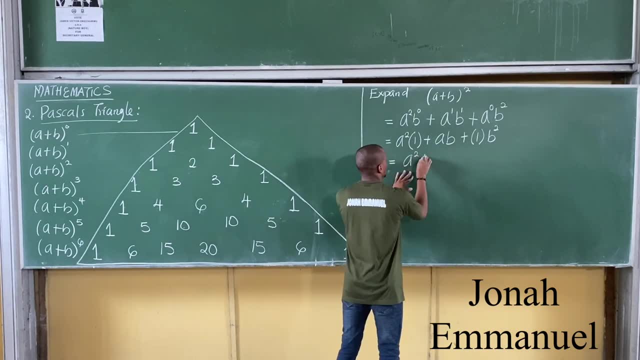 Plus a to the power 0 is 1.. And then I'm having b squared. So this gives you: equal to a squared times 1 is a squared. Plus a to the power b plus 1 times b squared is b squared. 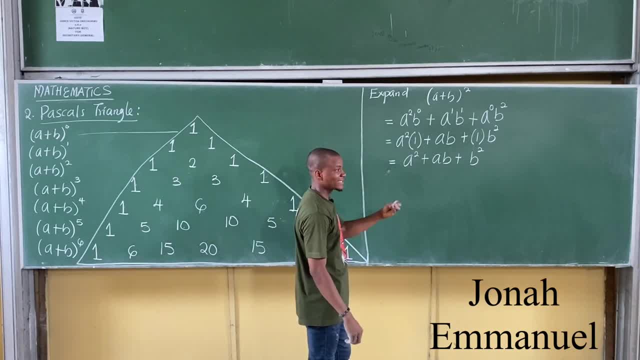 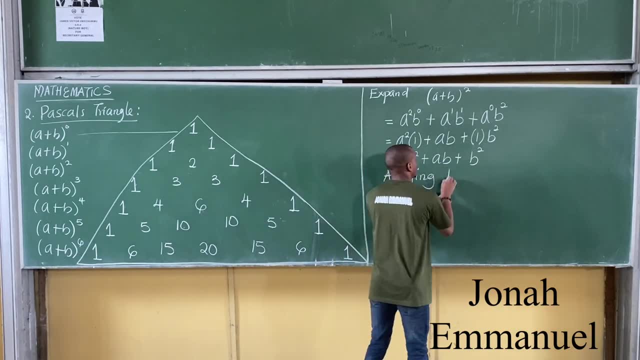 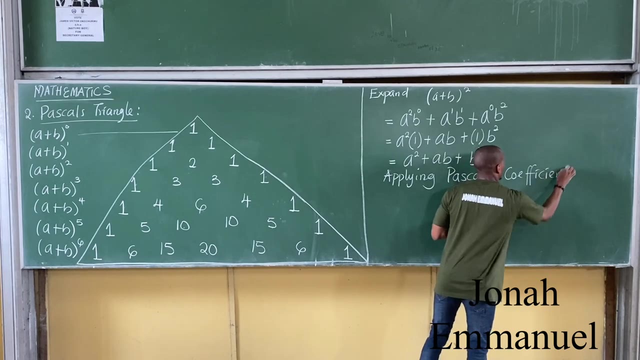 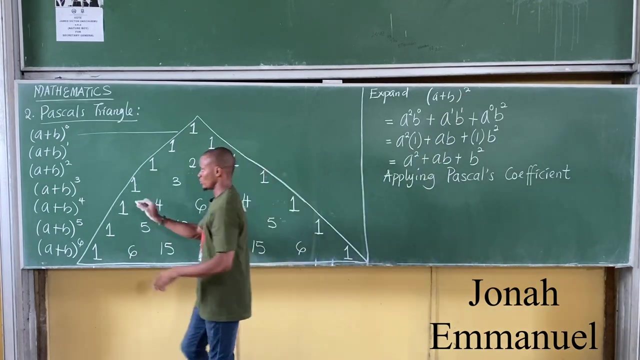 Now, at this point, you now apply Pasteur's coefficient. So, applying Pasteur's coefficient, the degree that I'm getting is the degree 2 over 2.. So I'll come to my Pasteur's triangle. That's this one here. 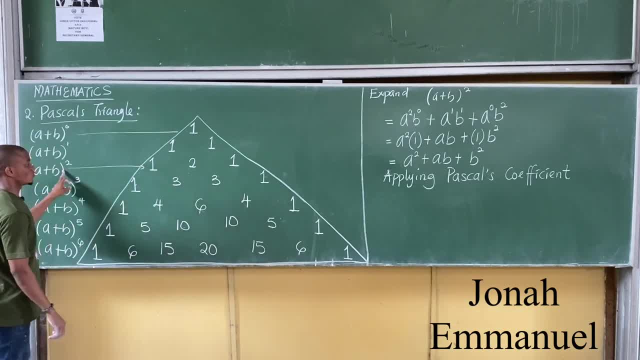 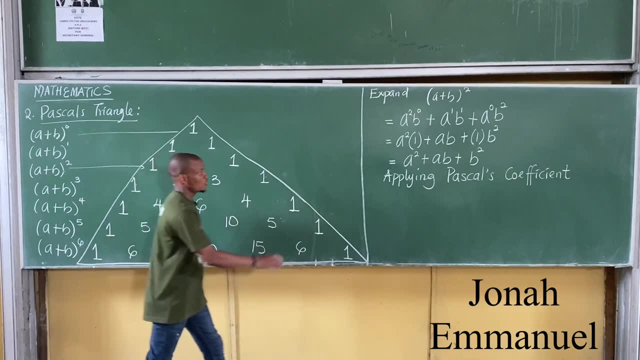 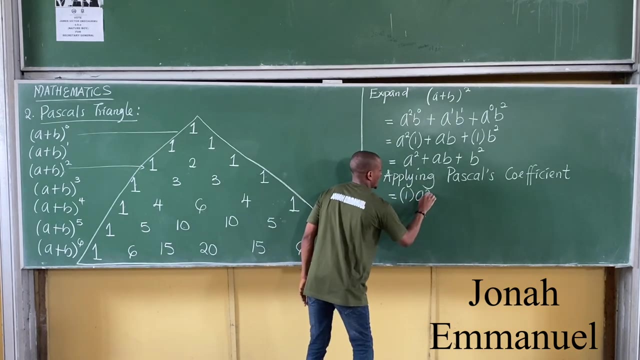 If I trace this, I'll have that for part 2.. My index is 1 to 1.. So this becomes the coefficient of each of the terms. So I'm having 1 to 1. The first one here. my equation is 1 into this a squared. 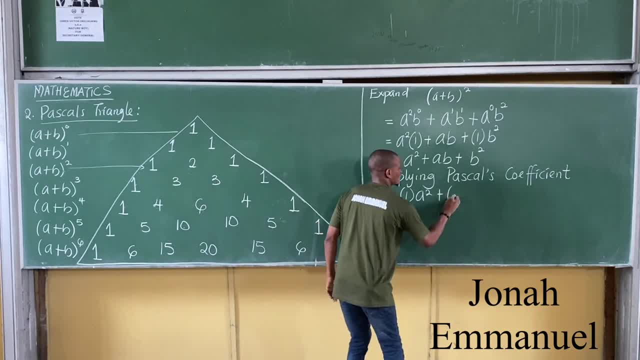 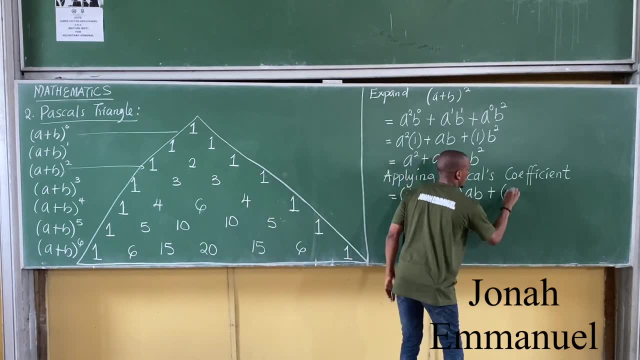 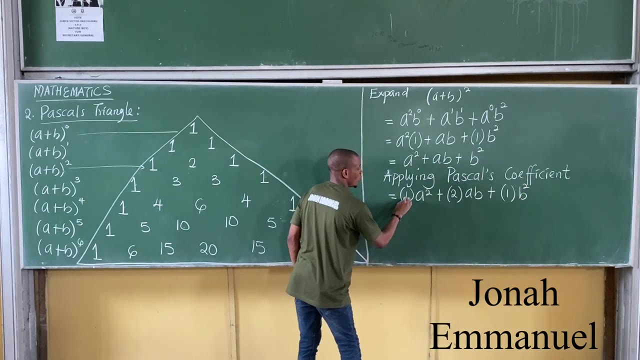 Plus we have 2 next. So it becomes 2 into this term here. That's a plus I have 1.. So I have 1 into this term here: b squared- Alright, so expand this. It becomes equal to 1 times a squared is a squared. 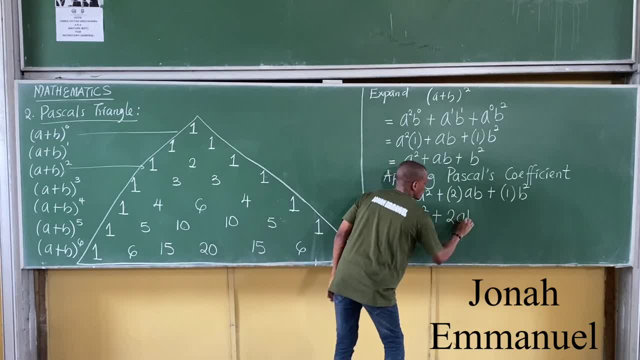 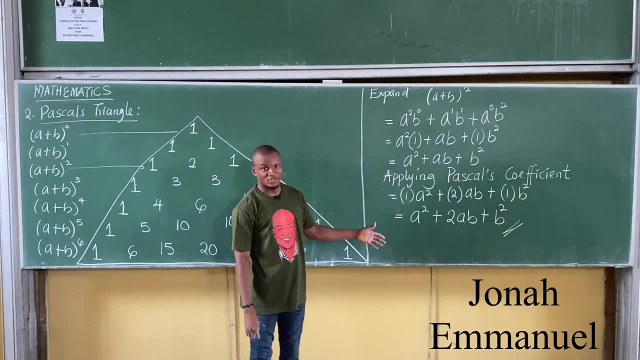 Plus 2 times a b is 2 a b. Plus 1 times b squared is b squared. So this is the answer of the expansion. Of course, this one is the same result we had when we did the general expansion method. 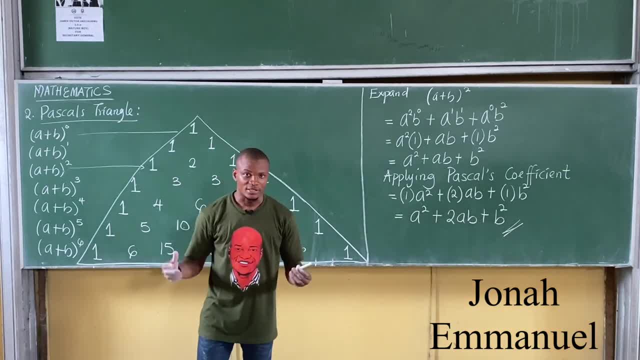 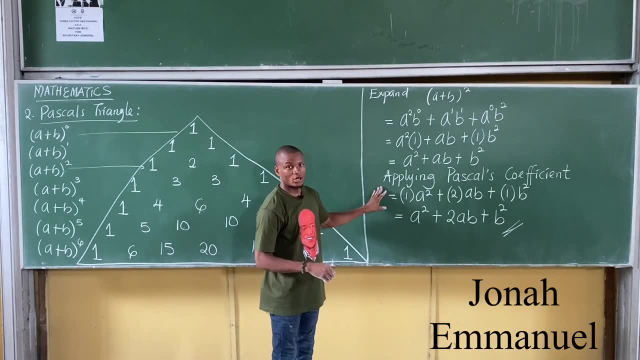 Alright, We'll take a second example and see how this works. Okay, so one last thing, please. The beautiful thing about Pasteur's triangular method of solving binomial expansion is that, using Pasteur's triangle, I don't have to collect like terms. 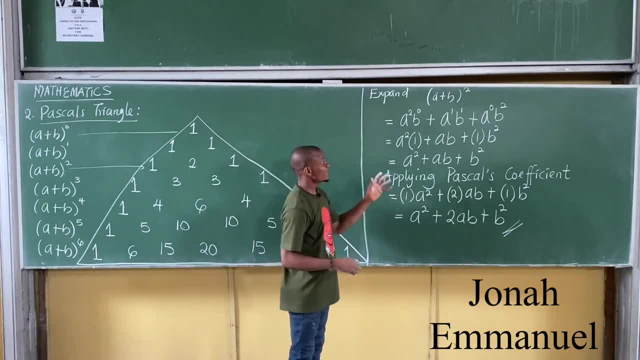 Alright. So if you observe here I don't collect like terms, Pasteur's triangle helps you to arrange the terms or arrange each term as it should be. That's like what's unique about Pasteur's triangular method. Alright, There's no collecting of like terms. 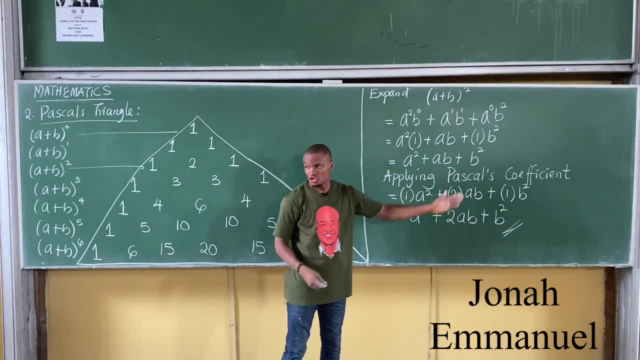 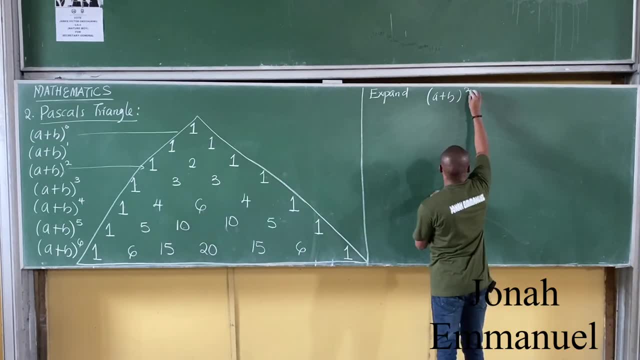 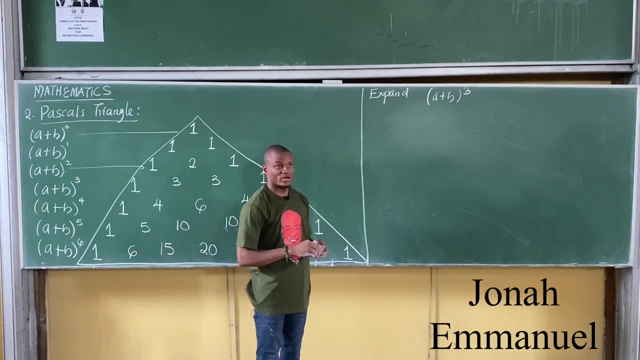 No, All the terms will arrange themselves accordingly. Just bring in their coefficients and then expand. That's all. Let's take a second example, Alright? So let's look at the second example on Pasteur's triangular method of expanding terms. So, when it comes to Pasteur's triangle, the first task is to raise the first term to all the parts. 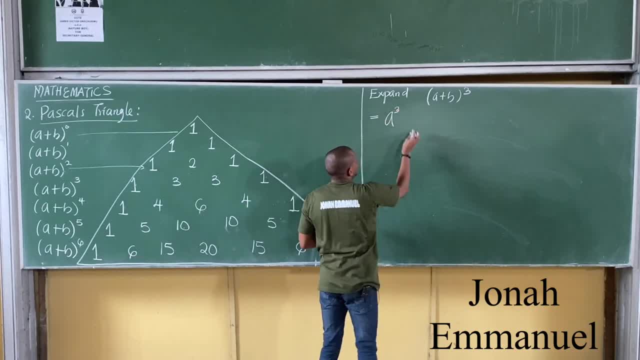 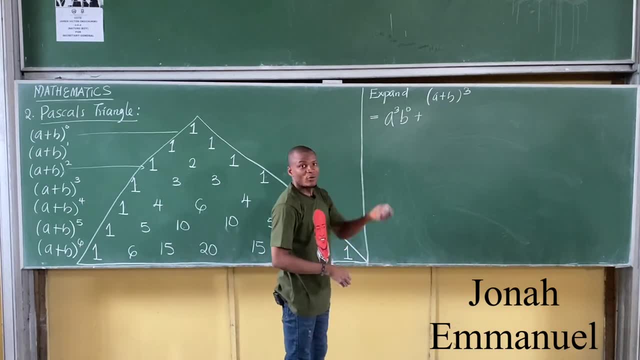 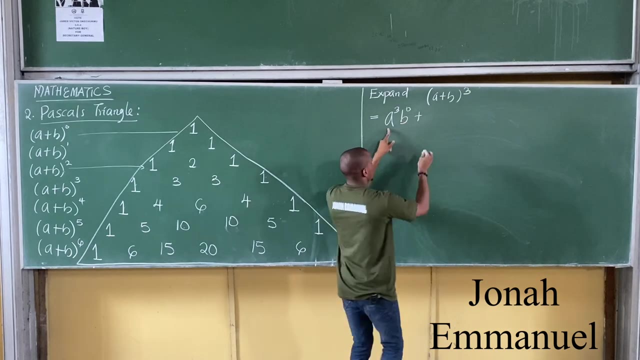 So it becomes a to the power 3, such that the second term is left with nothing, Plus my next term. I will reduce the power of the first term by 1.. I will increase the power of the second term by 1.. So it becomes a into this minus 1.. 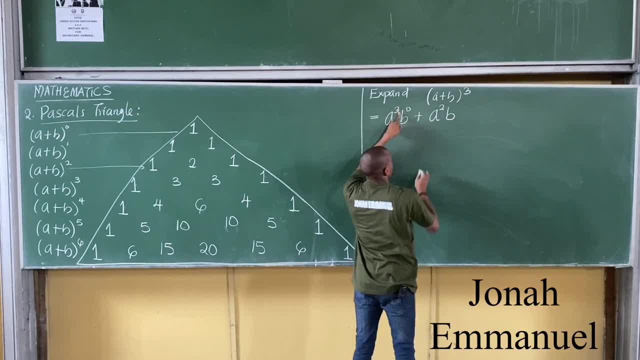 3 minus 1 gives you 2.. b into 0 plus 1 gives you 1.. Plus my next term. Reduce the power by 1.. Increase it by 1.. It becomes a. to the power: 2 minus 1 is 1.. 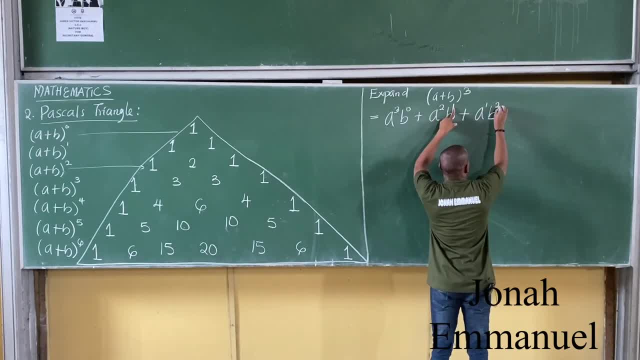 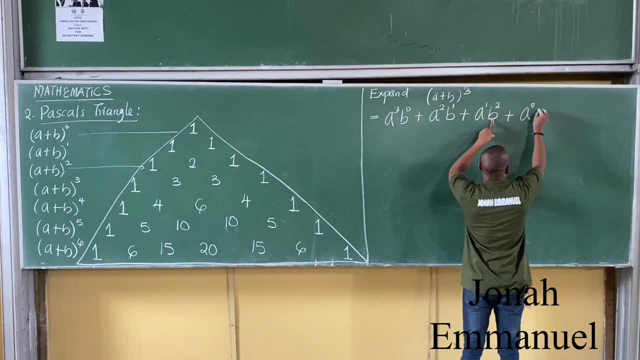 b into 1 plus 1 is 2.. Plus, I'm adding a: 1 minus 1 is 0.. Then b into 2 plus 1 is 3.. Obviously, at this point I will stop. I said you stop at the point where the first term is to the power: 0. 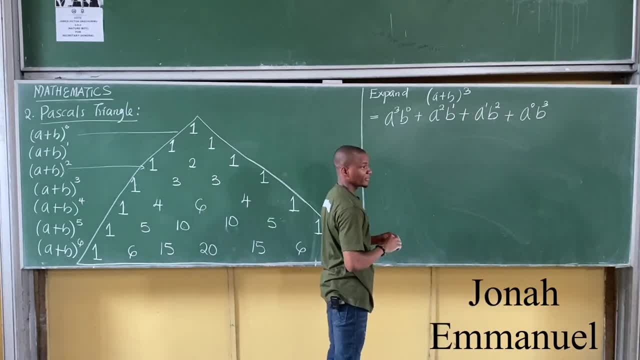 And the second term takes all the power. That's where you stop. Alright, so if you find this becomes equal to this: gives you a cubed b to the power. 0 is 1.. Plus, I'm adding a squared b to the power. 1 is b. 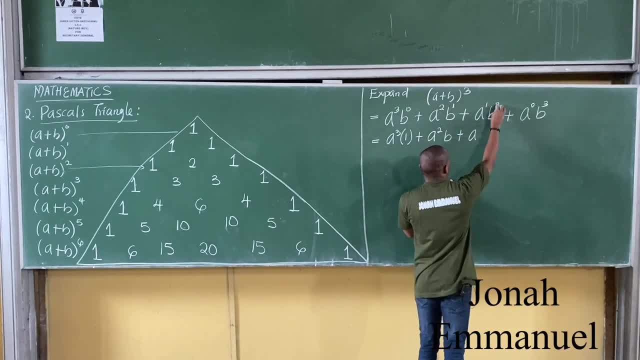 Plus a to the power 1 is a. Then next up, b squared. Plus a to the power 0 is 1.. Next up, I have b cubed. Alright, If I simplify further this times, 1 gives you a cubed. 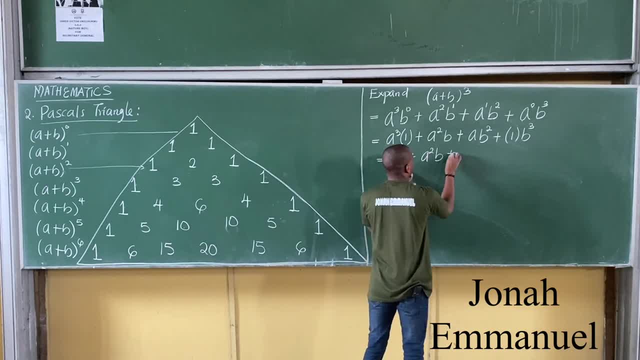 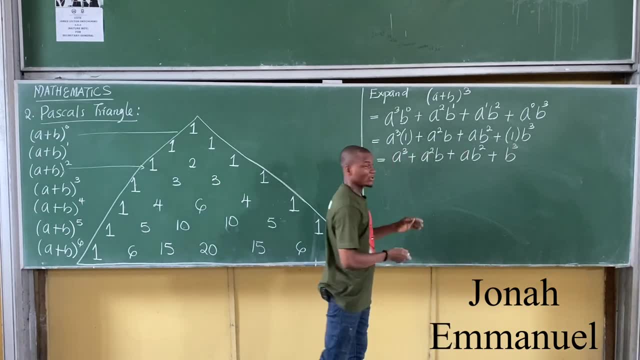 Plus this gives you a squared b. plus this gives you a b squared. Plus 1 times b cubed gives you b cubed. Observe, I don't have to start collecting like terms. The terms are already arranged. So what next? 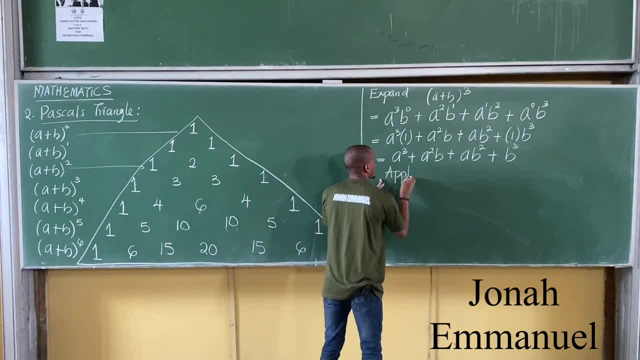 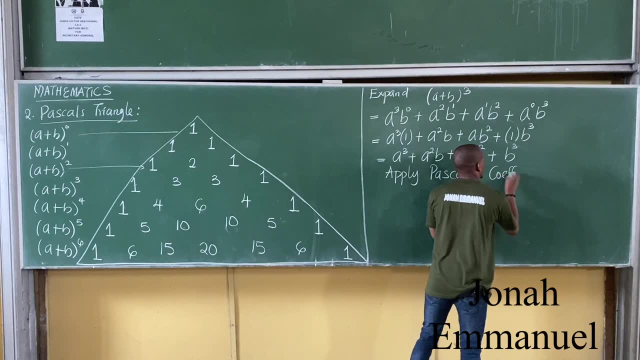 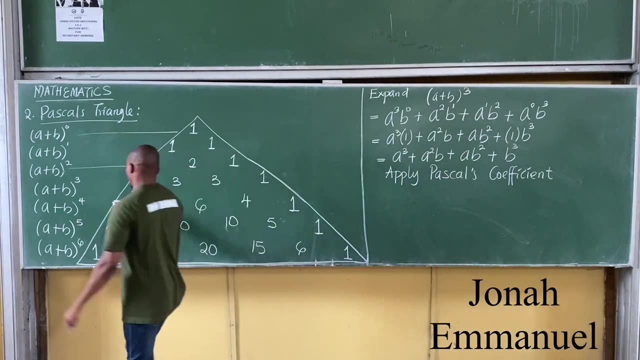 I will now apply FASTA coefficient. Apply FASTA, FASTA coefficient. If I look at the given degree into power 3. So from there to power 3. My coefficients are 1,, 3,, 3,, 1.. 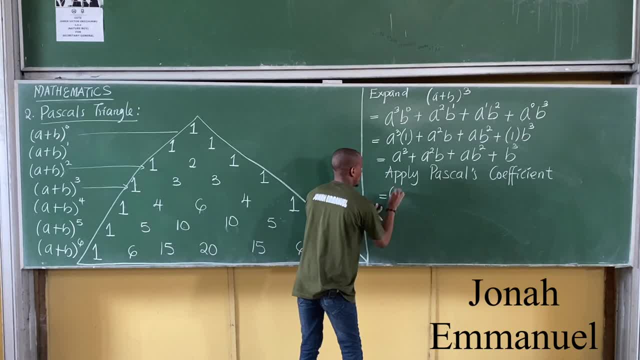 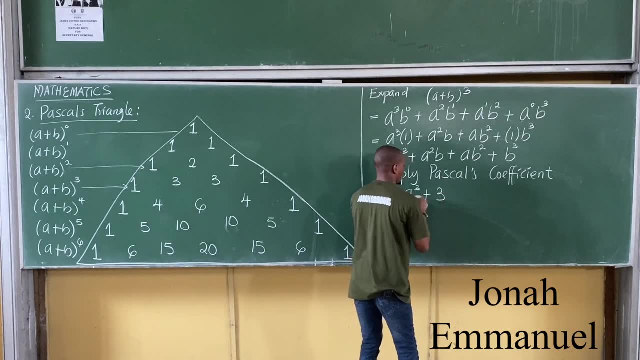 It becomes equal to To this one, I will add 1.. Then a to the power 3.. That's a to the power 3.. Plus for this I will add 3.. So 1, 3.. Attached 3 to this becomes a squared b. 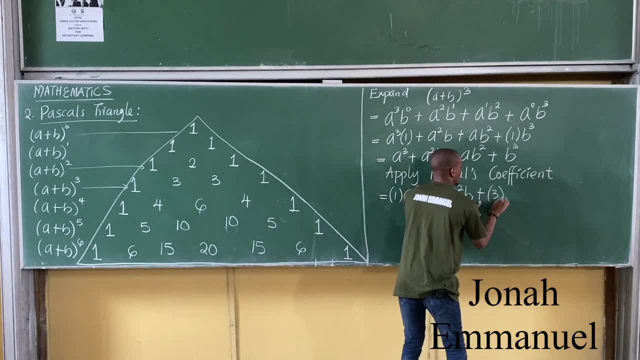 Plus attached 3 to this, 2 becomes 3 into a b squared, Plus 1 to this 1 b cubed. So I'm having 1,, 3,, 3, 1.. As my FASTA coefficient for degree 3.. 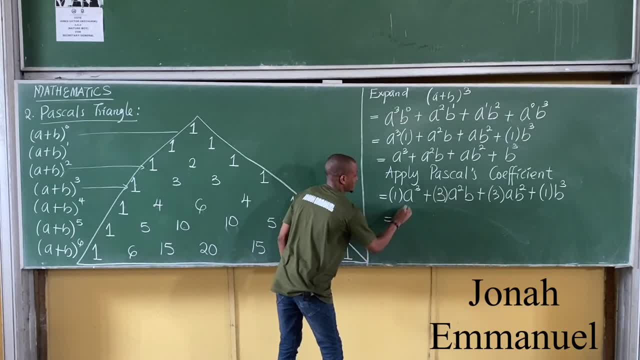 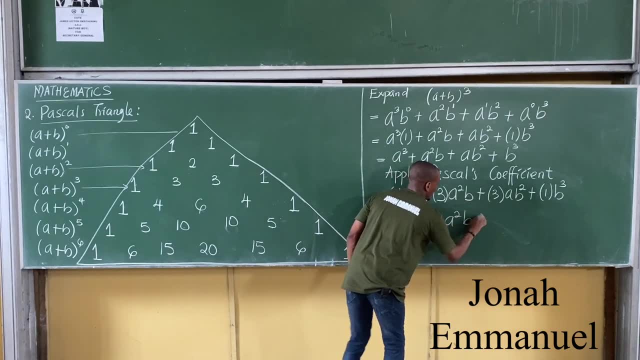 If I expand this, This is equal to this times: this gives you a cubed Plus this times: this gives you 3 a squared b Plus this times this 3 a b squared Plus 1 times this b cubed. 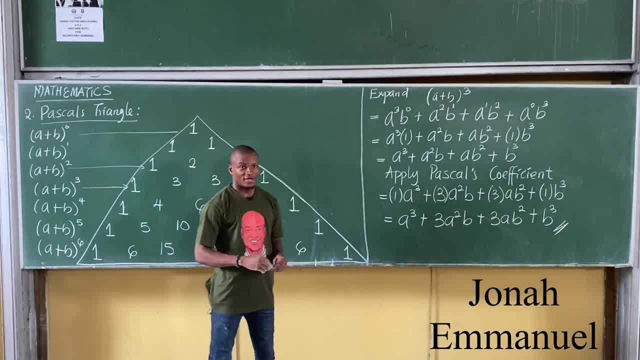 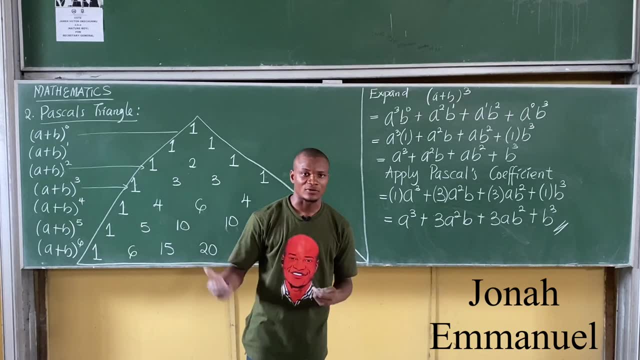 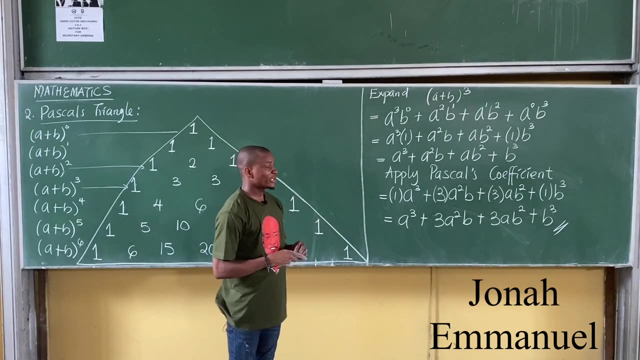 So I have this as the answer. after expansion: Alright, so we'll just do something. We'll see how to use FASTA triangle to do expansion for terms, Even without going through this lengthy process. Alright, We'll see how to use FASTA triangle to expand this. 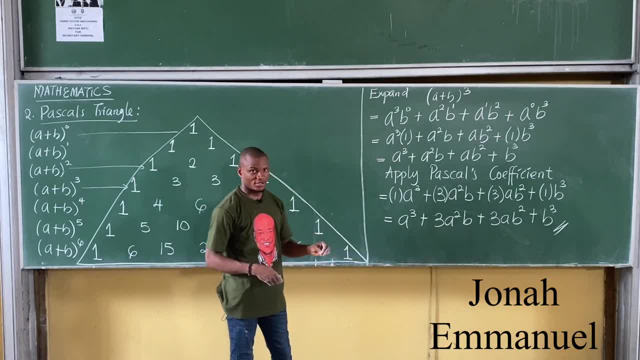 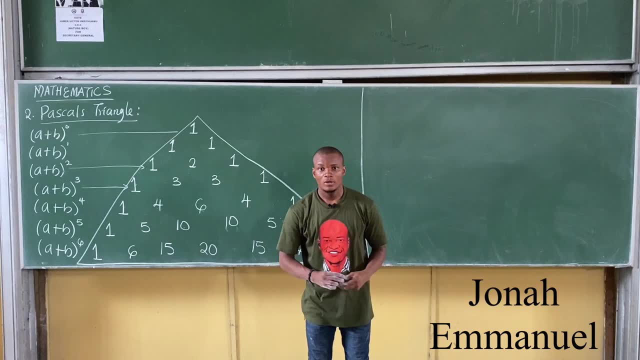 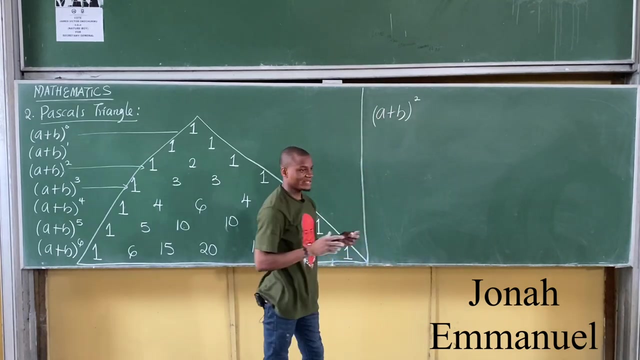 Even without going through this lengthy process. Alright, so let's look at a fast method of getting expansion without going through the whole complex method. Now let me start with what we did earlier. We said we had a plus b squared. Let's say I was to expand this using FASTA coefficient of FASTA triangle. 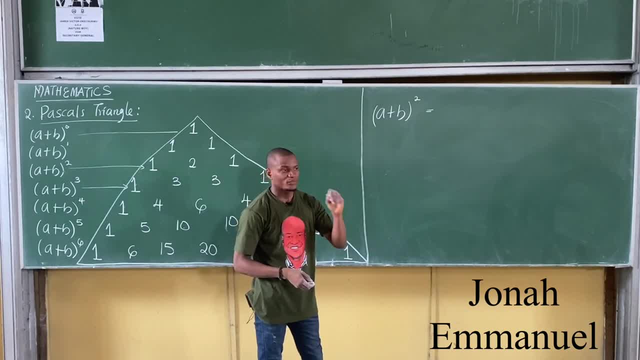 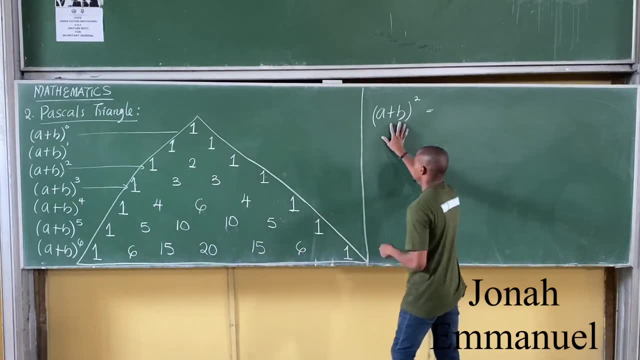 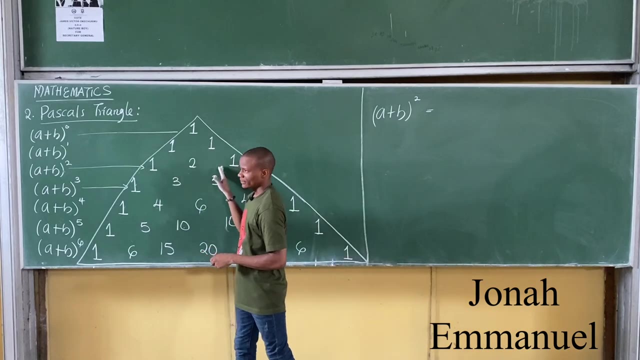 Without going through the lengthy process. What do I do Now? your first task is to always note the coefficient of the terms. Alright, For this, the index here is 2.. So for index 2, my coefficient is 1 to 1.. 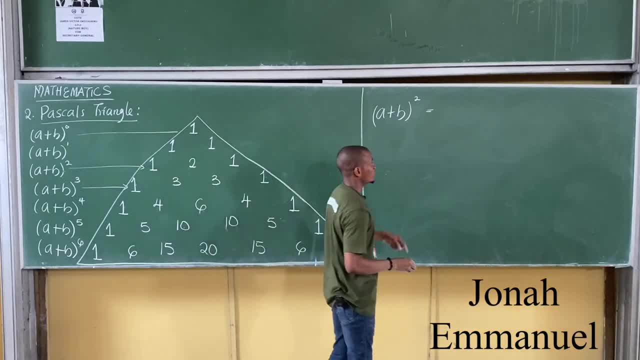 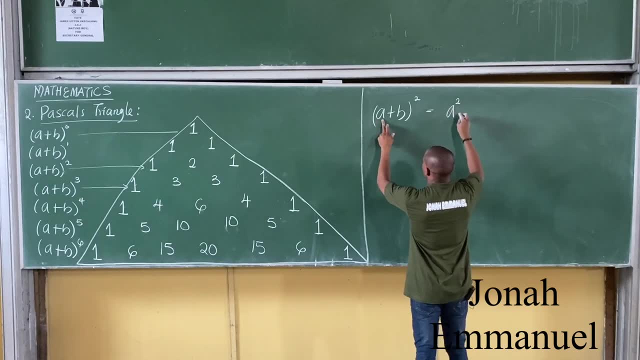 Alright, so bear in mind it's 1 to 1.. So how do I expand this? We said for FASTA triangle: this one takes all the power, So it becomes a squared. Of course. b to the power, 0 gives you 1.. 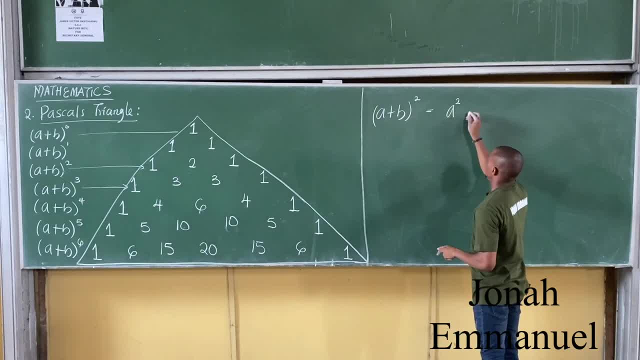 So the coefficient here should be 1.. So I'm having a squared Plus. my 3 is 1, 2.. So notice if I have 2. Into reduce this by 1. It becomes a to the power 1.. That's a. 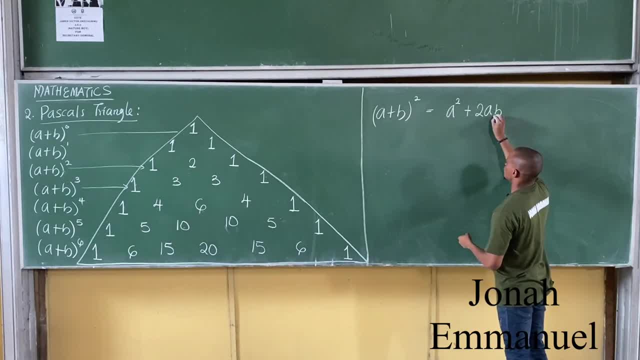 Increase b by 1.. It becomes 0 plus 1. Which is 1.. So I have b to the power 1, this Plus, finally, I have 1.. So it becomes a to the power 0.. 8 to the power 0 is 1.. 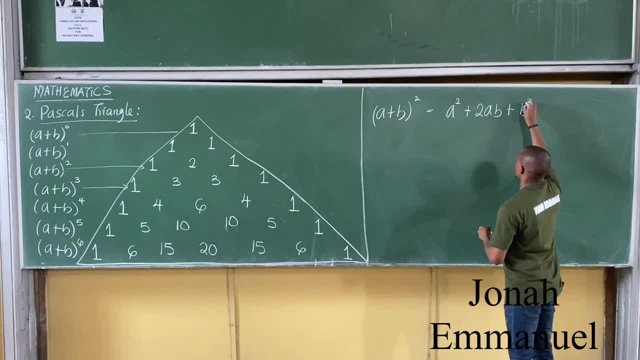 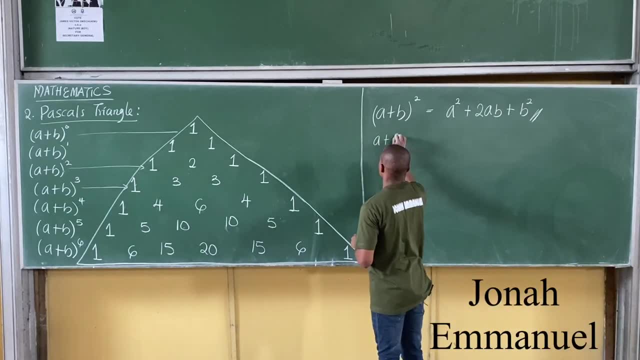 Then b to the power 1. there It becomes b squared. So this would be my answer: without solving, If I'm having a plus b to the power 3.. Without solving, How do I expand this? My concept would be: Note: the coefficient could be 3.. 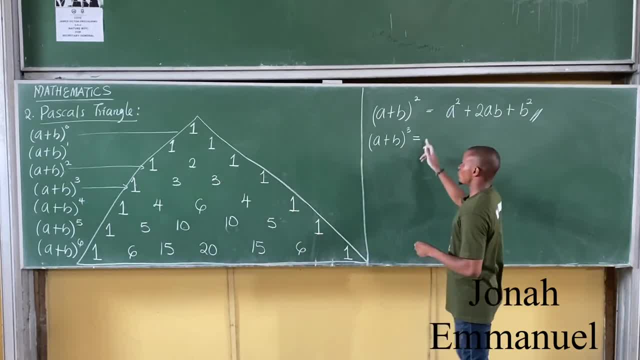 That's 1, 3, 3, 1.. So I'm starting off with 1.. Of course, 1 times anything is that thing. So I won't go there. I will take the first term, a, to the power 3.. 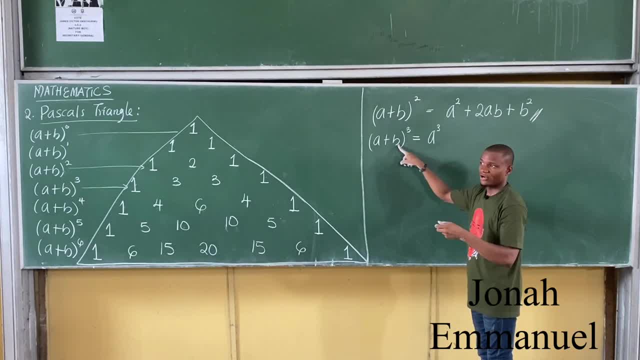 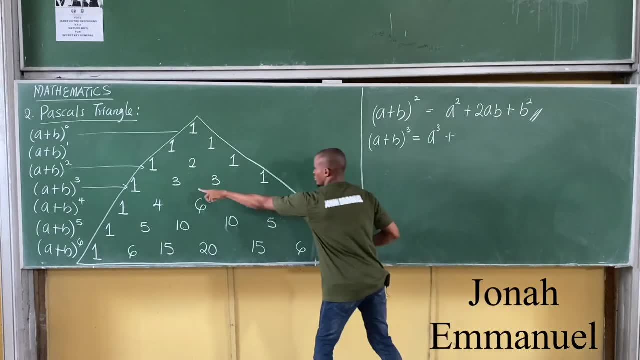 b is left to the power 0. That becomes 1.. From zeta of indices Plus instead is 1, 3, 3, 1.. My next coefficient here is 3.. So it becomes 3.. Reduce this by 1.. 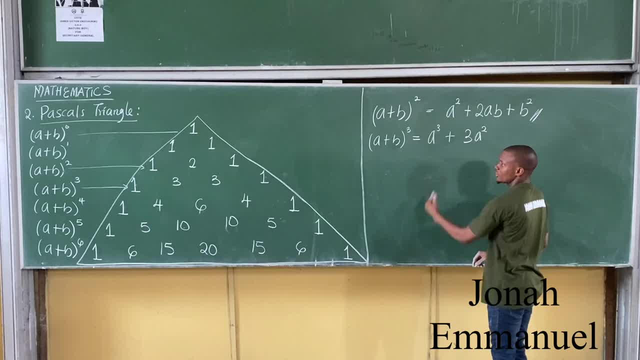 It becomes a squared b. here was 0.. Increase by 1. It becomes b to the power 1.. Which is b Plus. my next coefficient is 3.. Reduce this by 1. It becomes a 2. 2 minus 1 is what. 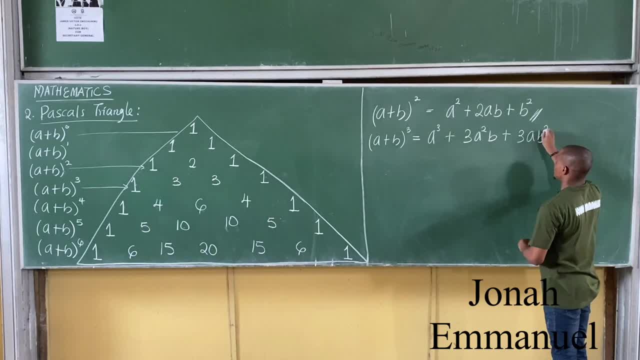 1. Increases by 1.. Because of that b squared Plus, finally I have 1. Into 8 to the power 0. Which is 1.. And then b cubed. So here is my final answer After expansion. 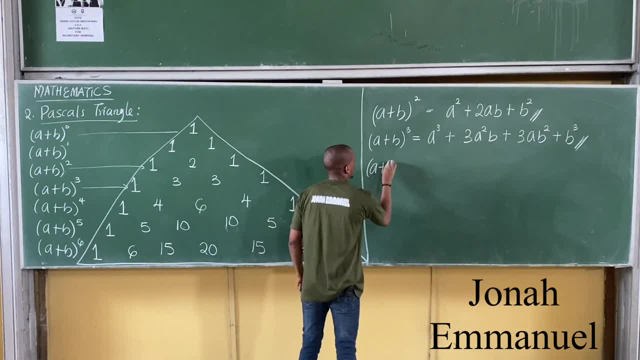 Let me take it to the fourth power point. Let's say I have a plus b to the power 4.. How do I expand this without going through the next process? It's simple. This would give you Of course For degree 4.. 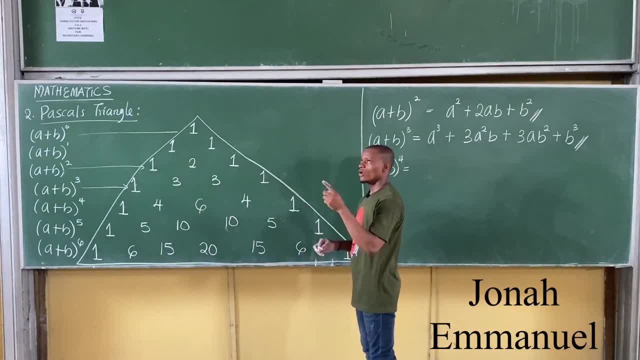 My equation is: 1, 4, 6, 4, 1. So I will note: 1, 4, 6, 4, 1.. So I will start with 1.. 1 times We said the first step takes all the power. 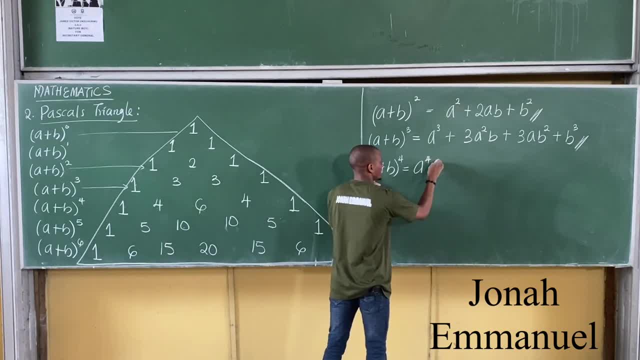 That becomes a to the power 4.. So 1 plus 4. This becomes a. Reduce the power by 1. It becomes 3.. b: The power here was 0. Increase by 1. It becomes 1.. 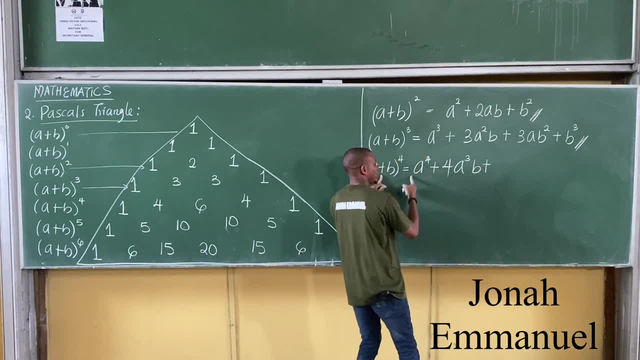 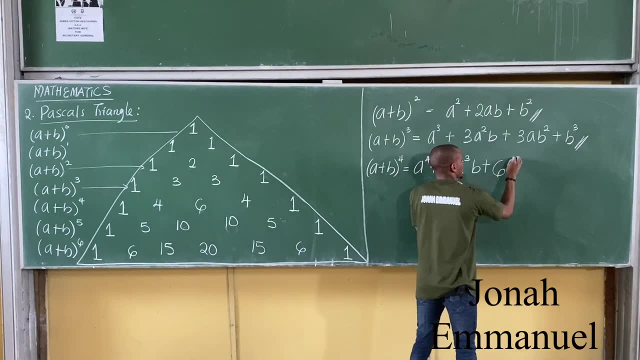 So I'm having this Plus 1, 4.. Next up is 6. It becomes 6.. Reduce this by 1. It becomes a squared. Increase by 1. It becomes b squared Plus. I'm taking 1, 4, 6.. 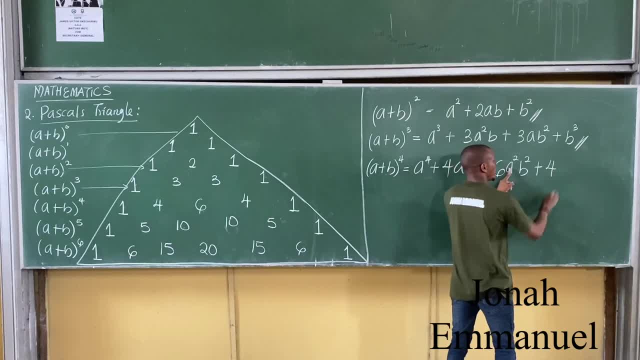 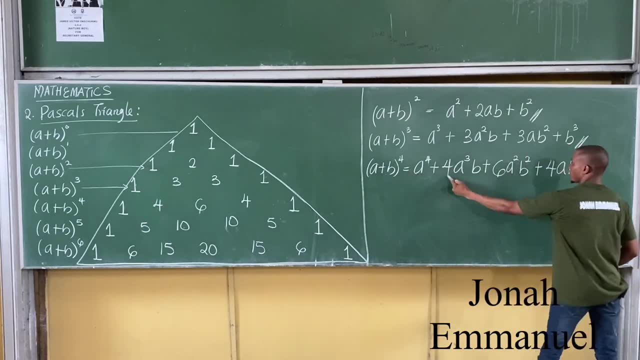 Next up: 4.. Reduce this by 1. It becomes a. Increase this by 1. It becomes b, cubed. So I have 1, 4, 6, 4 plus. Next up is 1. a. Reduce this by 1.. 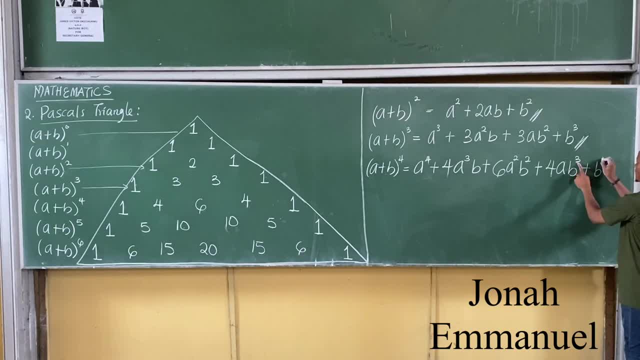 Gives you 0.. Increase this by 1.. Reduce this by 1.. Increase this by 2.. Increase this by 2.. Gives you 0.. Gives you b. squared, This becomes 1.. Which means this: b to power 4.. 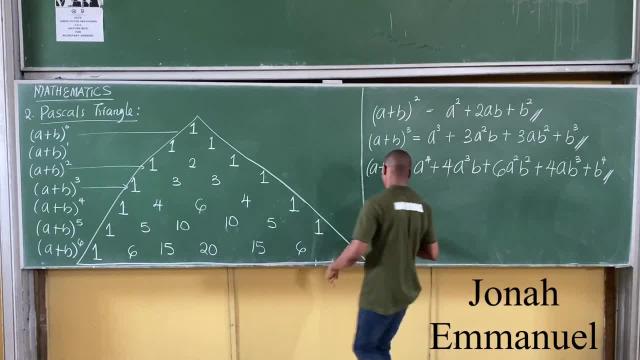 So I have. This becomes a shortcut for solving problems of volume expansion. Let's say I was asked to expand, for instance, X plus y to power 6.. Very fast, All these value To power 6.. My direction is 1,, 6,, 15,, 20,, 15,, 6,, 1.. 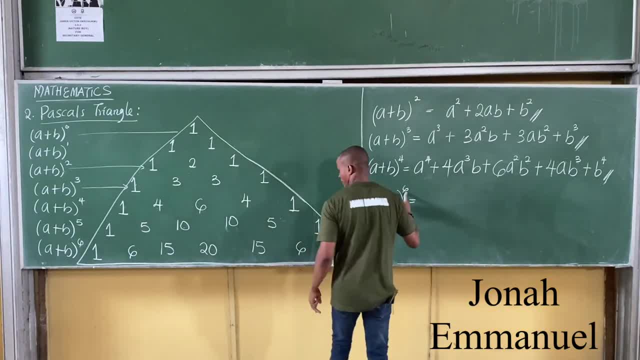 So it becomes: This is X power, 6. Plus I'm having 6.. So it becomes 6. 3. 6., So this becomes 6.. It becomes 6. 6.. So I have 4.. 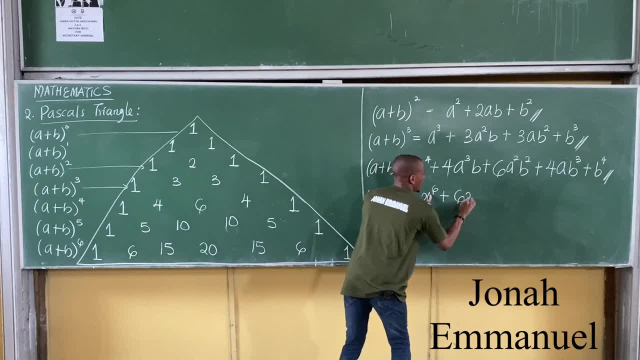 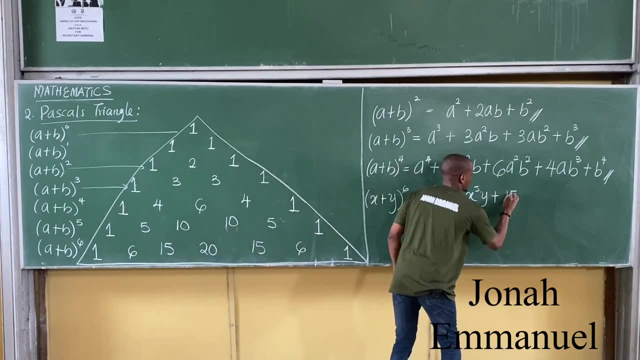 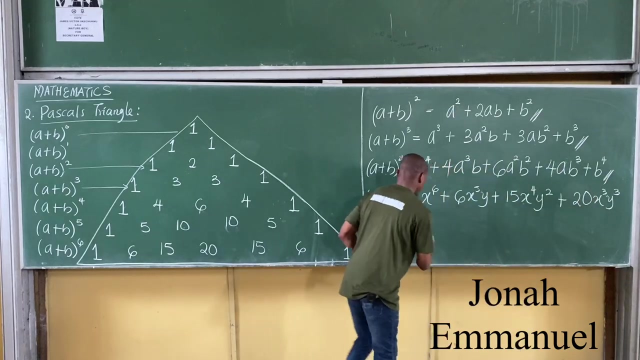 Just add up 2 times 6,. this reduced by 1, x to the power 5, y plus after 6,. next up is 15,. it gives you 15, x to the power 4, 1 squared okay- plus after 15,. next up is 20,. that gives you x to the power 3, 1 to the power 3, plus. 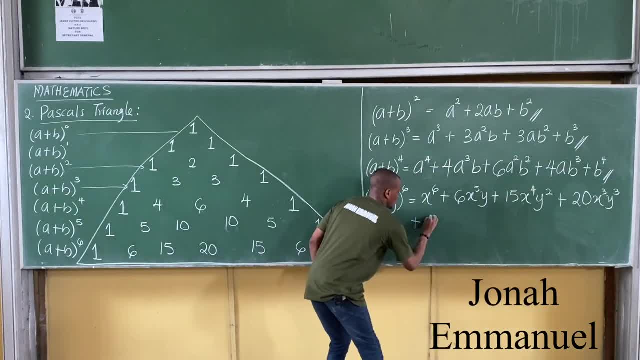 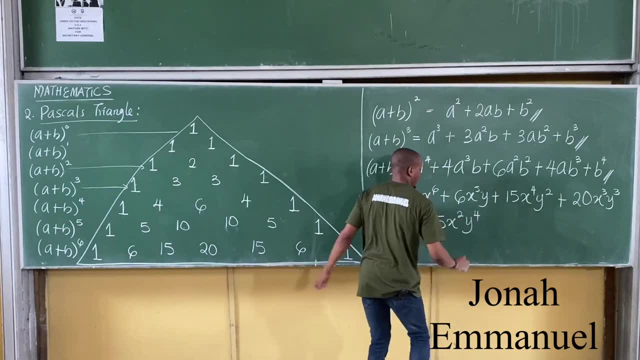 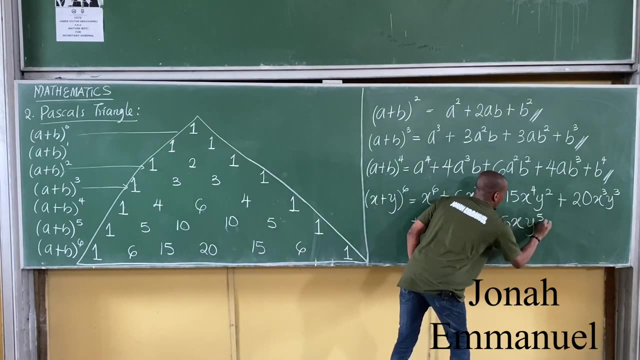 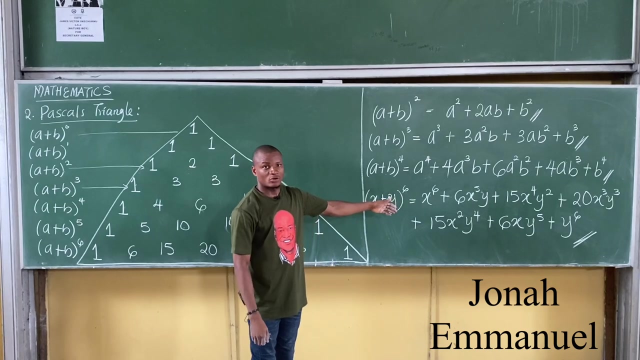 after 20, next up is 15, it gives you 15, x to the power 2, y to the power 4, next by 1, plus 6, into x to the power 1, that's x, then y to the power 5, plus 1 times y to the power 1, that's 6, so it's very easy to expand even without going to general methods. so this is how you solve problems using Pascal's. 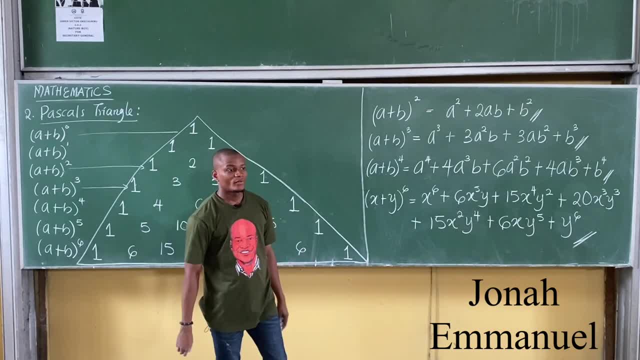 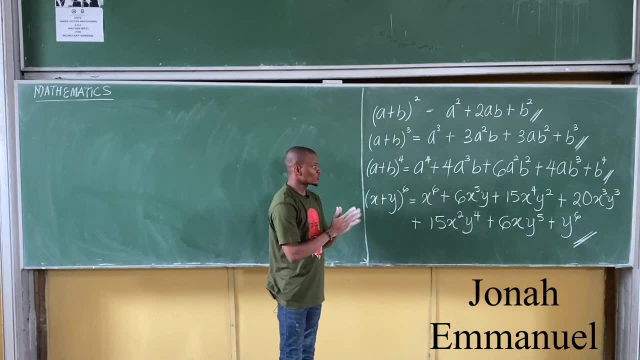 triangle method. okay, so I'm done doing my expansion. have I shown that my terms are correct? Now here's how to easily recognize that your terms are correct. if your terms are correct, the sum of the parts of each of the terms will be equal to the given part for this one here. let's look at this: the given part here is 3,. the power here is 3, for this term, because 2 plus 1, that 3,. 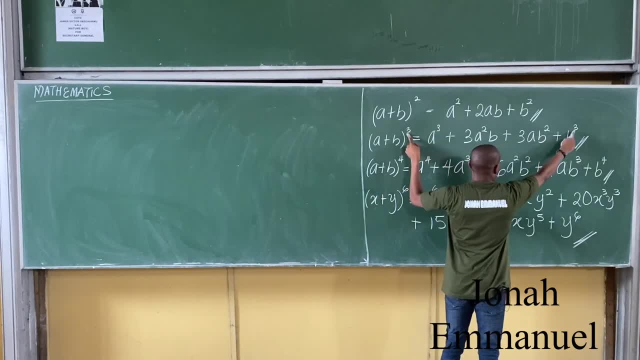 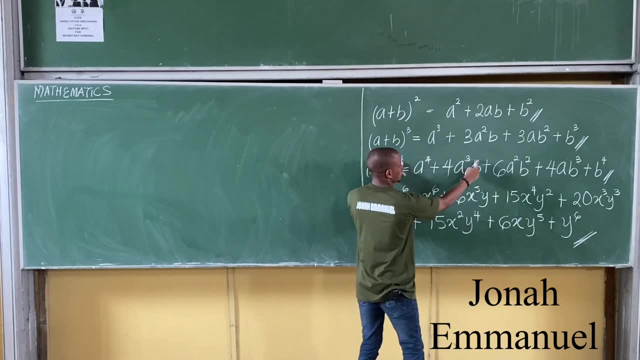 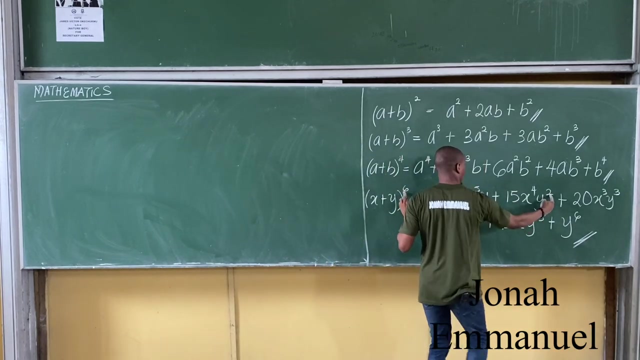 1 plus 2, that's 3,. 3 here, that's 3, for this term. this one here given part is 4, this term here has power 4, 3 plus 1 gives you 4,. 2 plus 2 gives you 4,. 1 plus 3 gives you 4, to power 4, this to power 6, I got 6,. 5 plus 1 gives you 6,. 4 plus 2 gives you 6,. 3 plus 3 gives you 6,. 2 plus 4 gives you 6,. 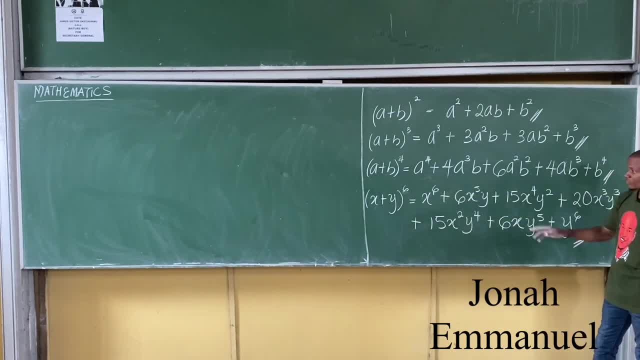 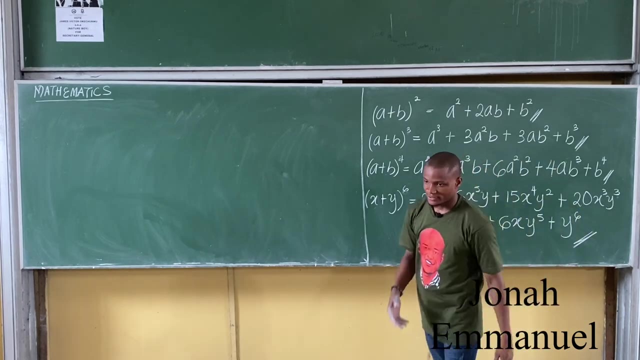 1 plus 5 gives you 6, and, of course, to power, 6,. so one way to confirm that your answer is correct is that if I do the sum of the parts of each of the terms, it will be equal to my given part. that's how to confirm that your answer is correct. alright, so in the next class we'll look at the third method of binomial expansion, called the combination method. alright, let's look at. 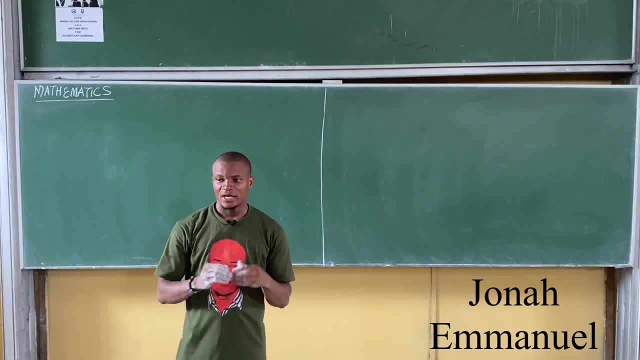 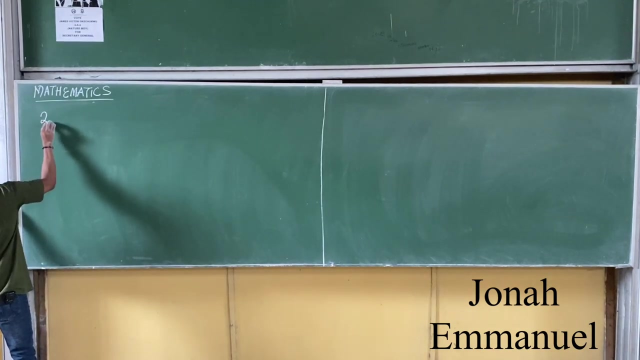 let's look at one more problem called Pascal's triangle. in our previous examples, the sign in between the terms are usually positive. so what happens if I have a negative term? what happens if I have a more complex term than just A and B? how do I evaluate it? let's take, for instance, a maximum evaluated value of, let's say, 2x minus 7y. 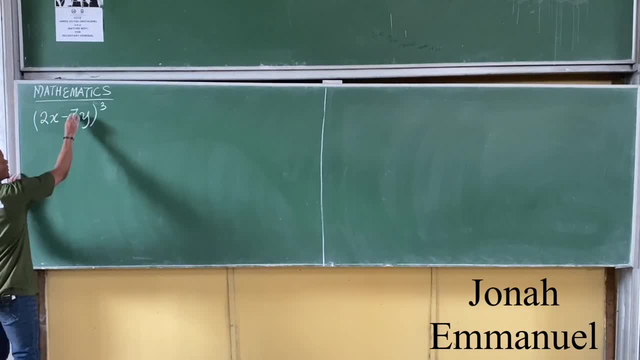 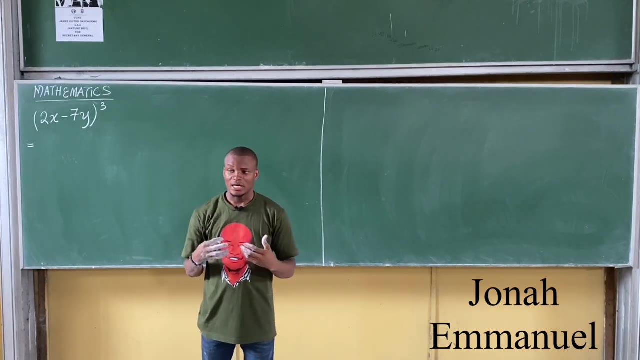 3, alright. so what is the maximum value of this using binomial expansion? what value? alright, at this point. choose any convenient method for you. as for me, I'm working with Pascal's triangle. I think that's the best for me, so I work with Pascal's triangle. when it comes to Pascal's triangle, or degree 3,, my coefficients are what there? 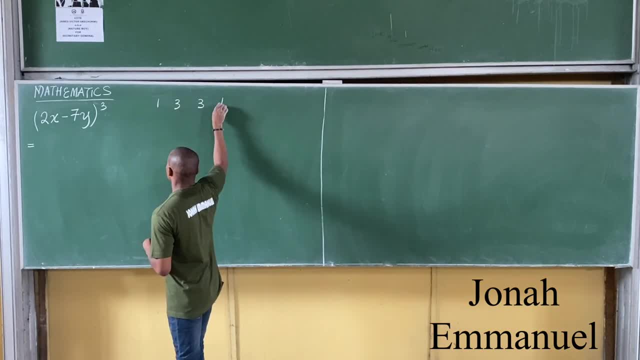 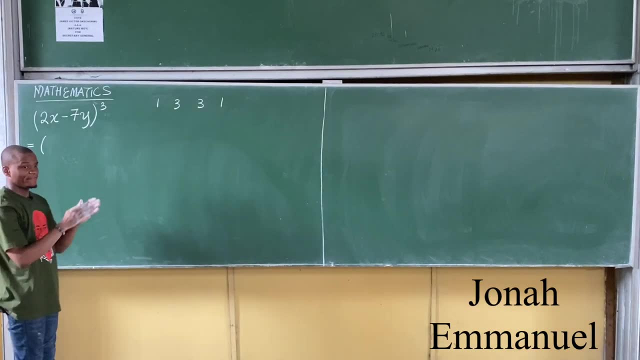 1, 3, 3, 1, so not this. alright. so what's the idea there? we said for expansion such as this, we said the first term takes all the part. my first term here is now 2x, not just x. so we come to 2x, so 2x here, first term takes all the part, that's 3,. second term: that's minus 7y. 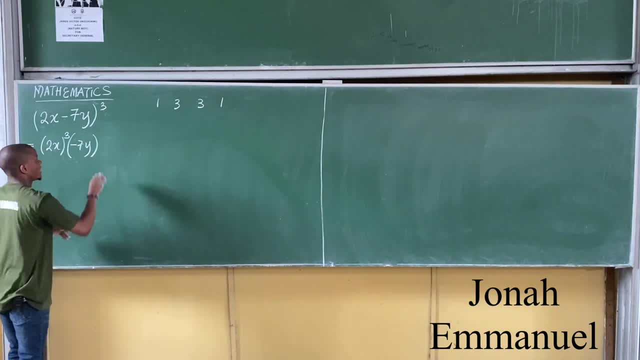 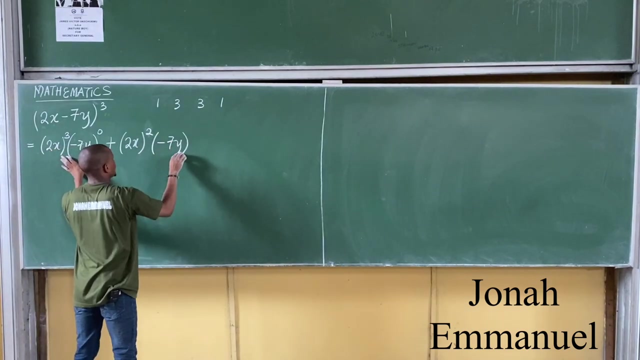 minus 7y is less than or equal to nothing. that becomes 0, plus the same concept. I will reduce the part here by 1,. I will increase the part here by 1, so it becomes 2x to the power 1, or 2, that's 3 minus 1 is 2,. next up, minus 7y to the power 1,. increase by 1, plus reduce by 1,. 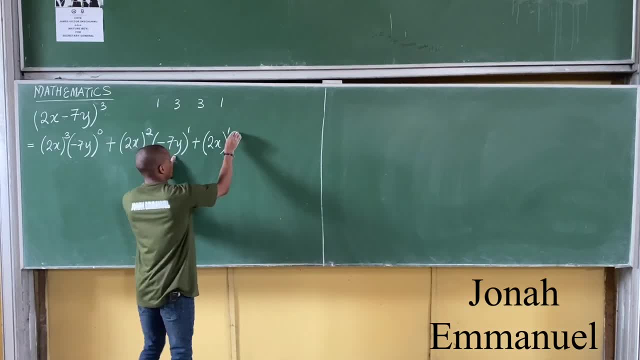 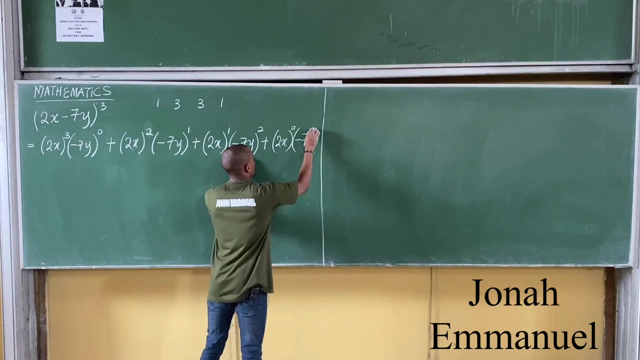 becomes 2x to the power 1,. increase this by 1, becomes minus 7y to the power 2,. finally, reduce this by 1, becomes 2x to the power 0, and the last term here- becomes minus 7y to the power 3, so it happens alright. 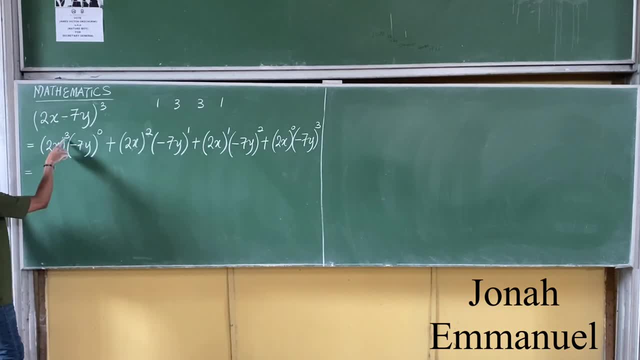 so in the 5, this gives you equal to. so 2 to the power 3 gives you 8,. next up, x to the power 3, gives you 8x to the power 3, this to the power 0 gives 1, plus 2 squared gives 4, now, mind you. 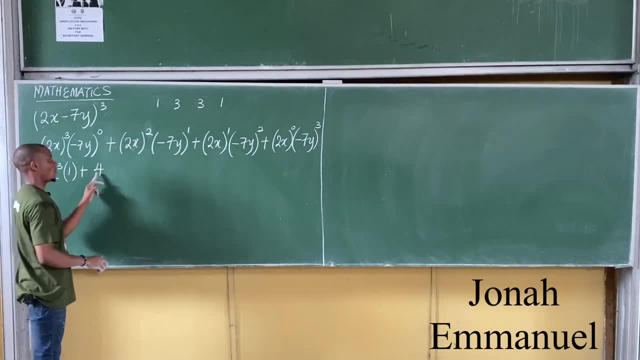 this 1 affects each of the terms. alright. so 2 squared gives 4, this idea gives x squared, this to the power 1 is 8x. alright, any term to the power 1 is that same term becomes minus 7y. 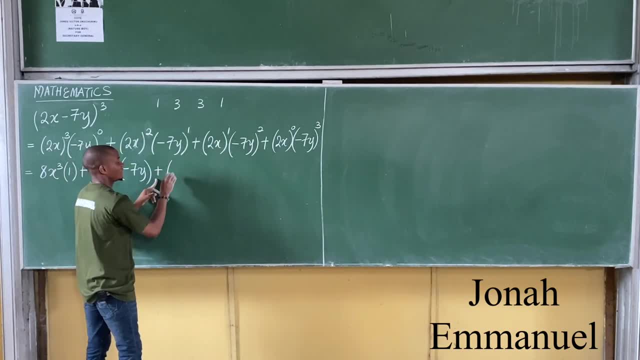 plus this to the power 1 is 8x, as we said earlier. next up: minus 7 squared minus 7y all squared. of course the squared affects the minus. so minus times minus is plus 7, squared is 49y squared. 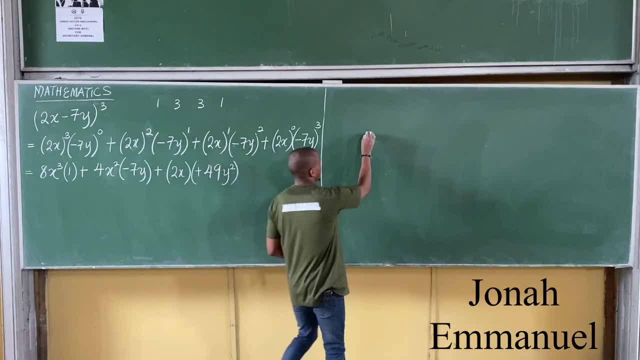 alright, if you are unsure of this. if you just come here and see minus 7y times minus 7y, minus 7y times minus 7y. alright, if you are unsure of this, if you just come here and see minus 7y times minus 7y. 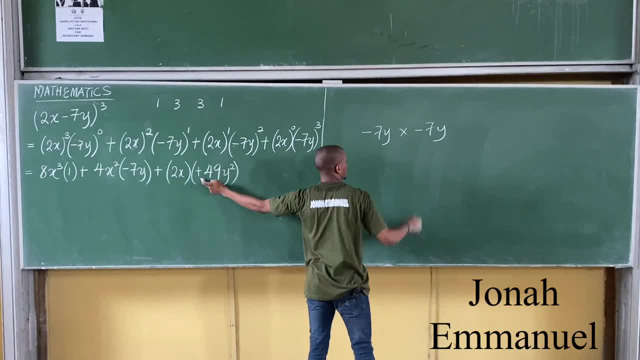 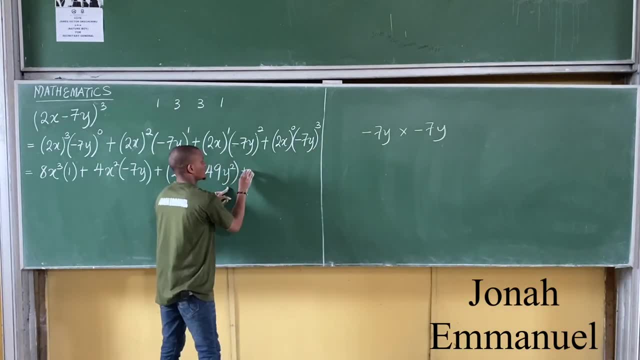 minus 7y times minus 7y minus times. minus is plus 7 times 7 is 49, y times y is y. squared plus this to the power, 0 is 1,. finally, minus cubed means minus times, minus that's plus, times minus that's minus. 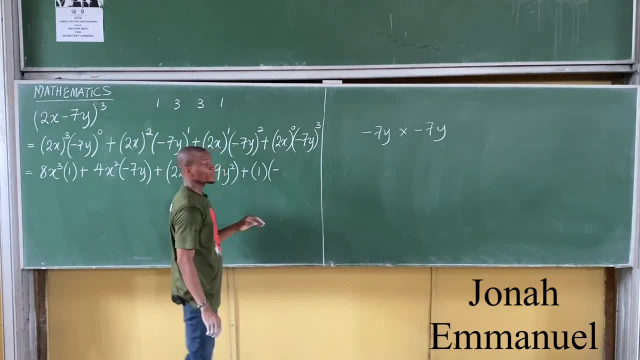 so minus cubed is minus 7 cubed. you see what 7 cubed is, what 7 cubed, 7 cubed, 7 cubed 3,, 4,, 3, next up, this one is y cubed. alright, so expand this. this is now equal to: 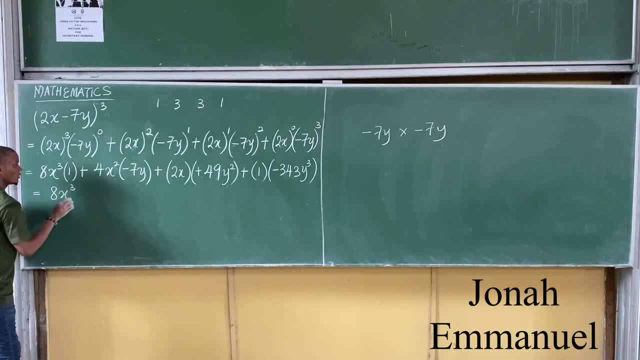 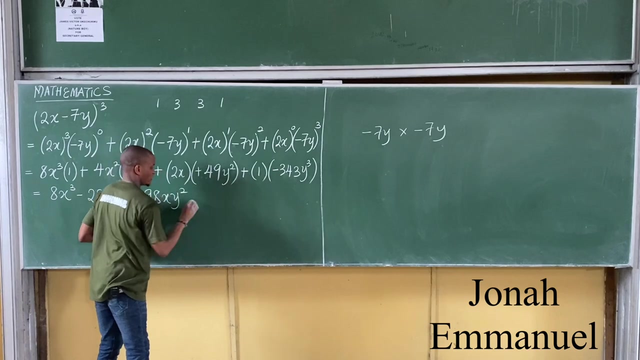 this times 1 is y. ok, plus minus is minus 7 times 4 is 28,. x squared y. x squared y plus 2 times 49 is 98,. this and this x- y squared plus times minus is minus 3,, 4, 3, into y cubed. so I have this: 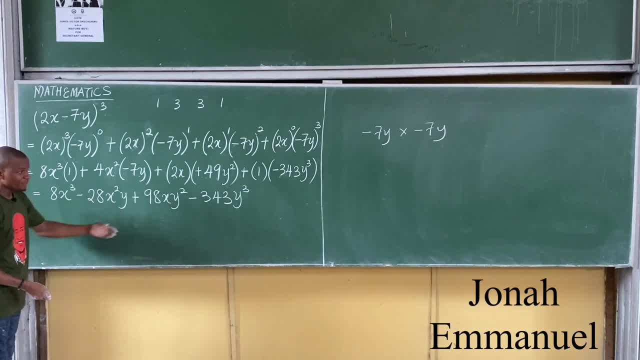 Now, this is my value after expansion. I have not yet included Pascal's coefficient. so after expanding it now, let's now apply. so applying Pascal's, Pascal's coefficient, let's apply Pascal's coefficient for degree 3, we said the coefficient is 1,, 3,, 3, 1,. 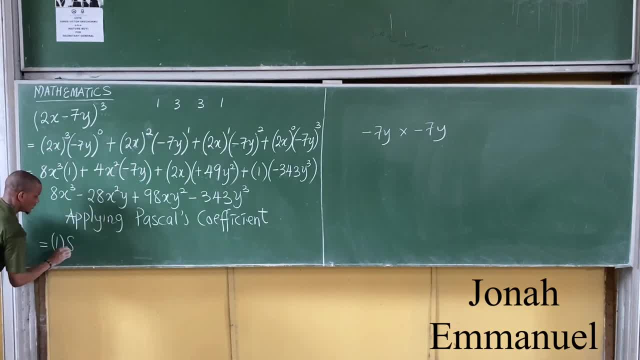 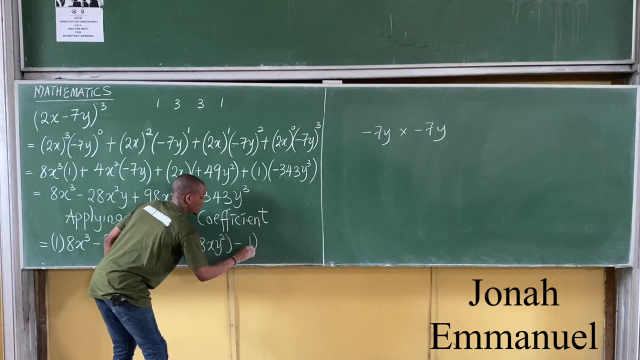 so it becomes 1, to the first term, 8x cubed minus 3, to the second term, 28x squared y plus 3, to this end here 98x xy squared minus 1,. so this is it here: 3, 4, 3, 1, cube. 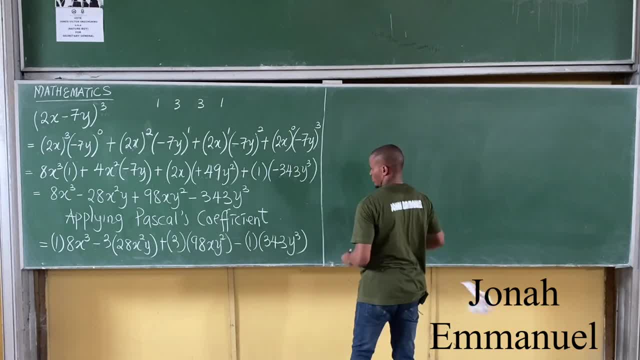 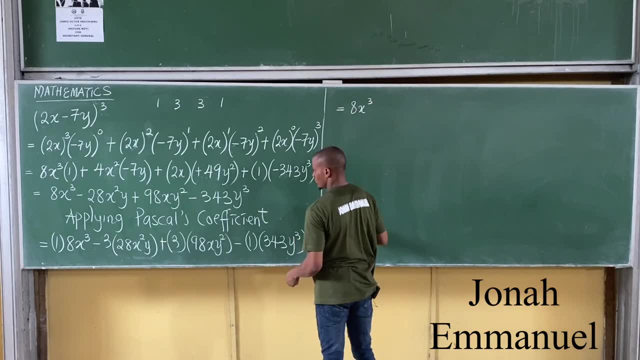 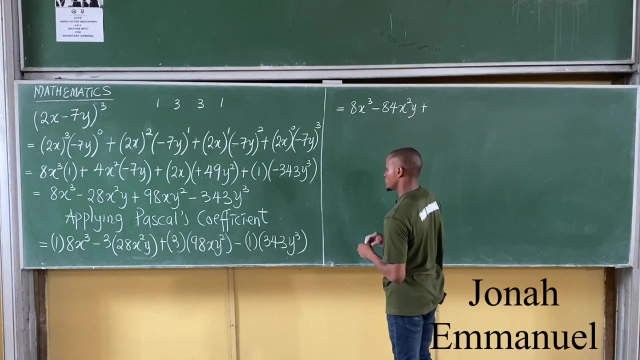 So I have my answers here. This is now equal to 1 times 8x cubed, is 8x cubed minus 3 times 28 is 84.. 84 x squared y plus 3 times 98 is 294, 294 xy squared. xy squared minus 1 times 3, 4, 3 is 3, 4, 3,, of course, y cubed. 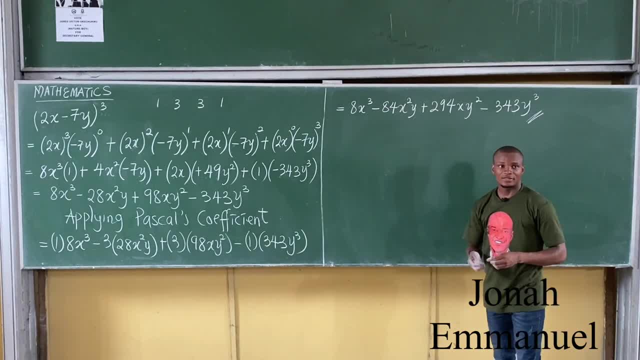 So this becomes the answer After the expansion. I have this, So this is how we solve problems using Pascal's expansion.